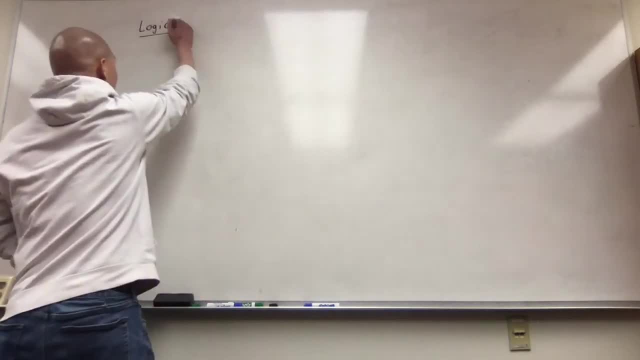 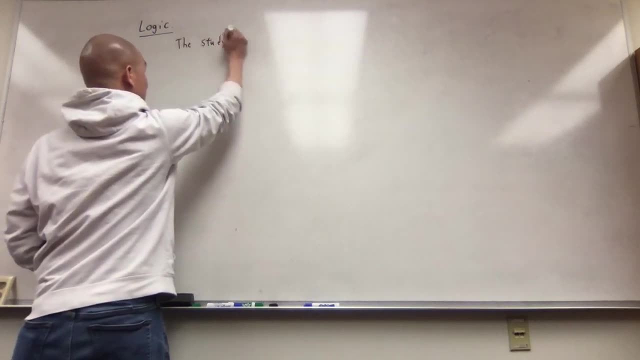 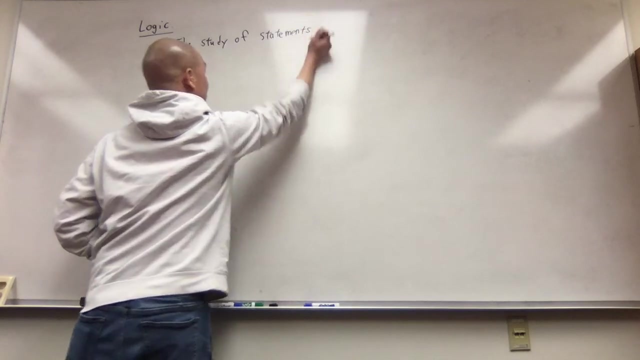 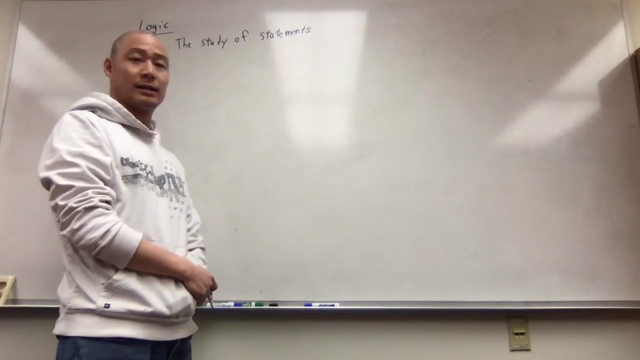 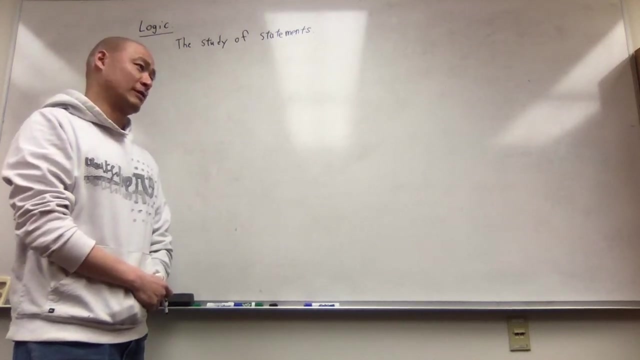 handout Now. logic is the study of statements and really at the very central heart of mathematics, this is what we study in math. Most people think that mathematics is the study of numbers or functions or operations of numbers, but that's really not, as a mathematician, what we do. 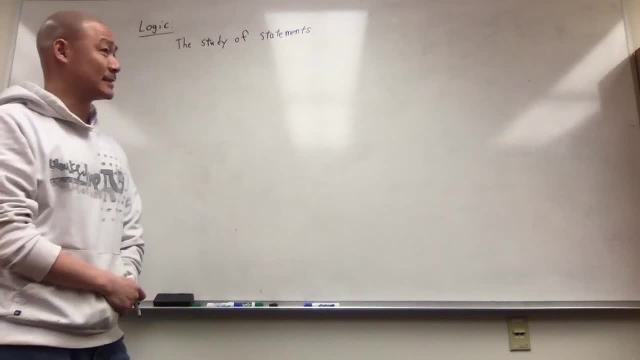 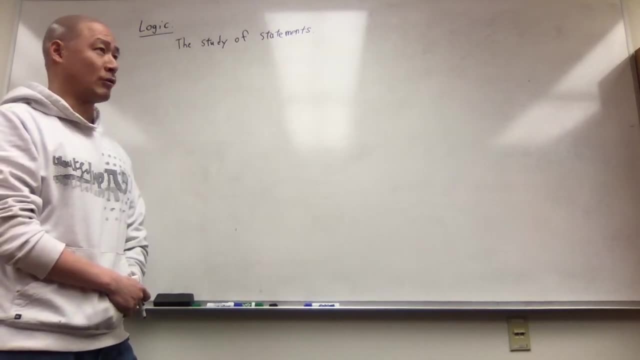 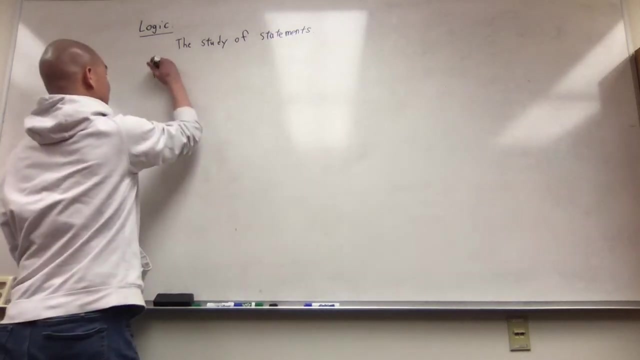 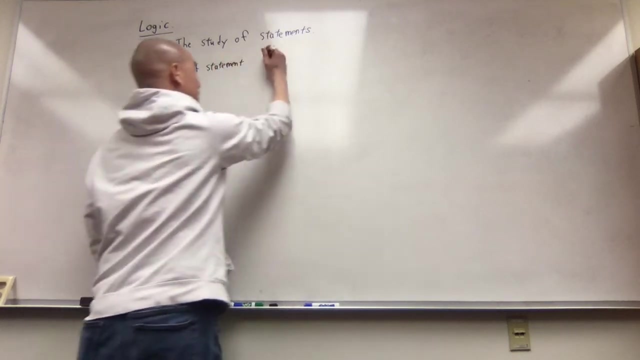 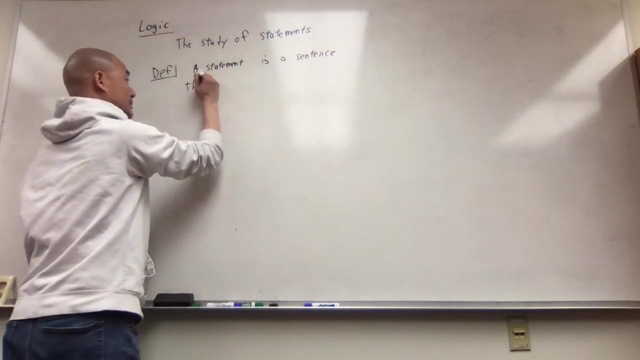 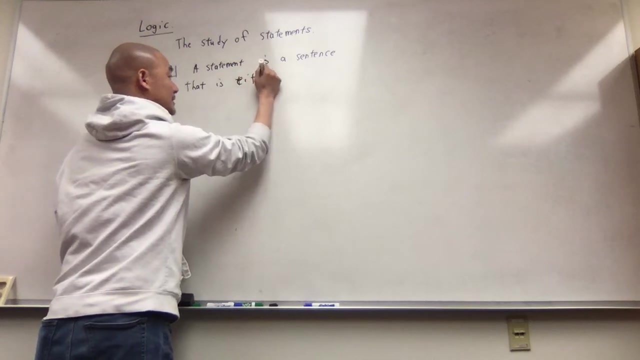 at all. What we really do is study statements, and very often, of course, these statements involve numbers or operations between numbers, but they're not the central focus. it's the statements that are the focus. So a statement is a sentence. that is either true or false. 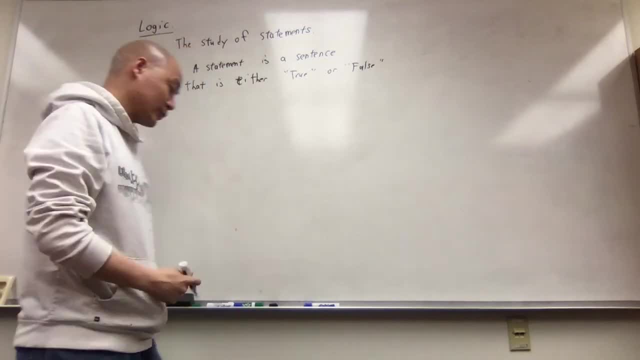 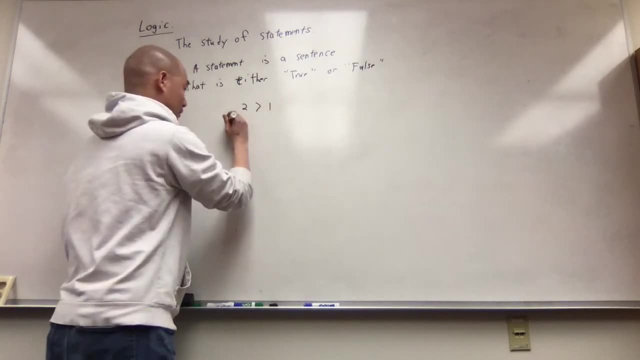 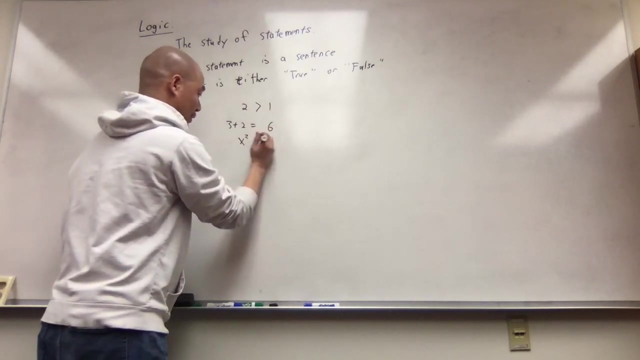 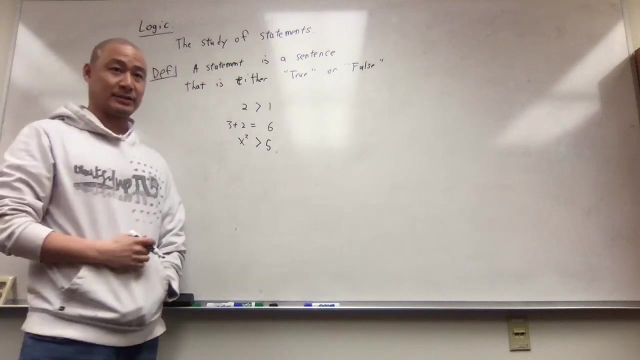 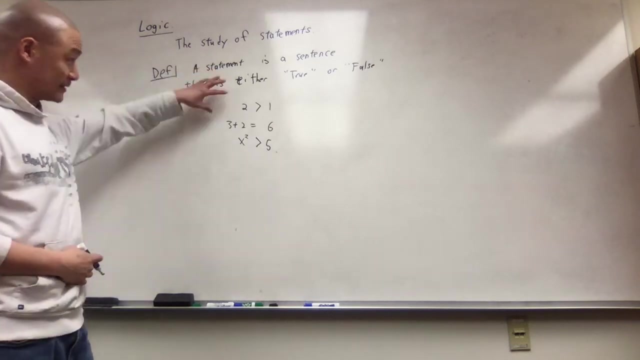 And so some examples of statements will be something like this: like: 2 is greater than 1, 3 plus 2 is equal to 6 and x squared is bigger than 5. so here are some examples of statements that use numbers that we might be used to. so some of these things- 2 greater than 1, for example- is a true. 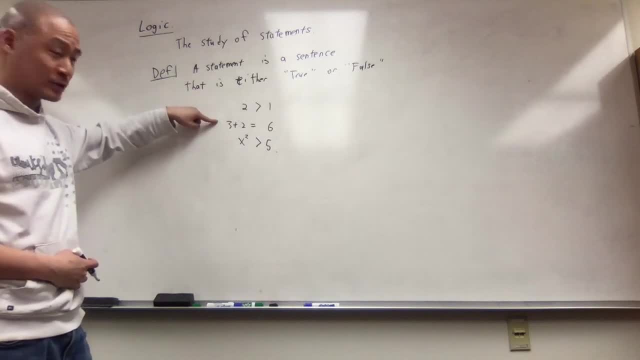 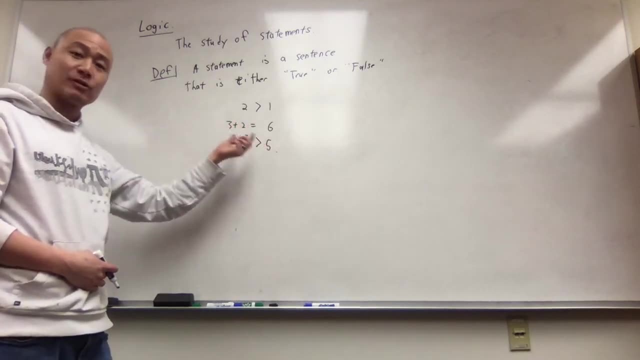 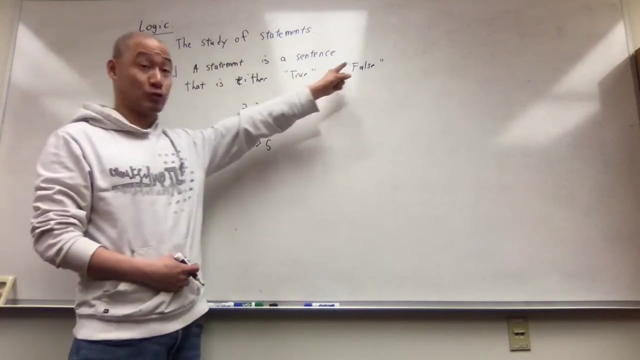 statement 3 plus 2 equals 6 is a false statement and x squared is greater than 5 is either a statement that's either true or false, depending on what X is. but the point is that for any value X, it would either be true or be able to be. 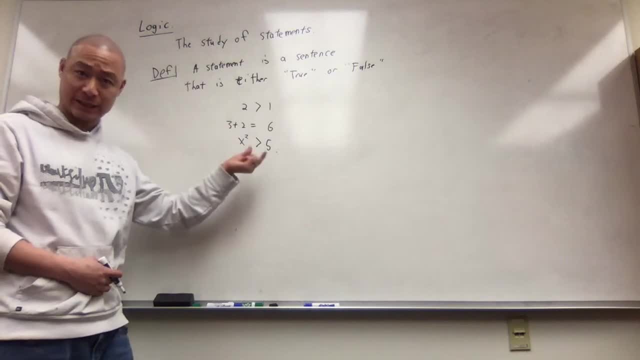 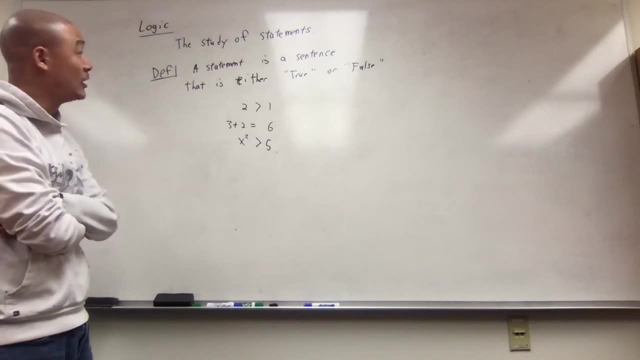 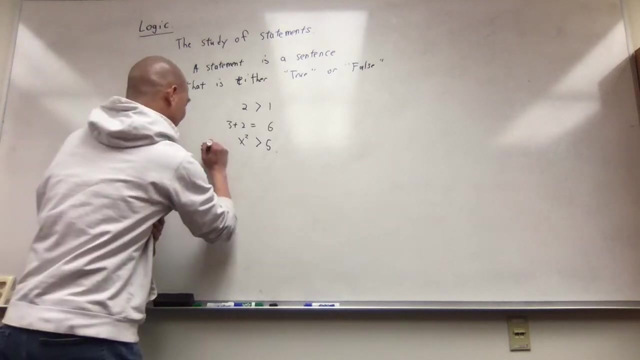 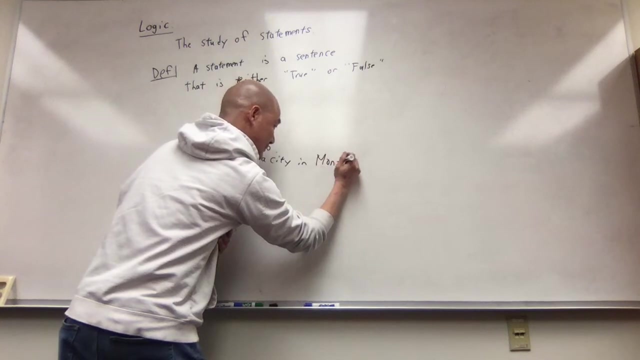 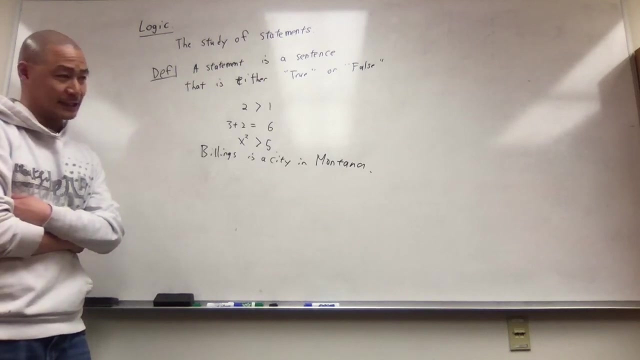 false, that it couldn't possibly be both or neither in any given circumstance. so a statement is any sort of sentence that is either true or false and, like I mentioned, we don't have to limit ourselves to just statements about numbers. Billings is a city in Montana. it's certainly a statement and it is certainly takes on. 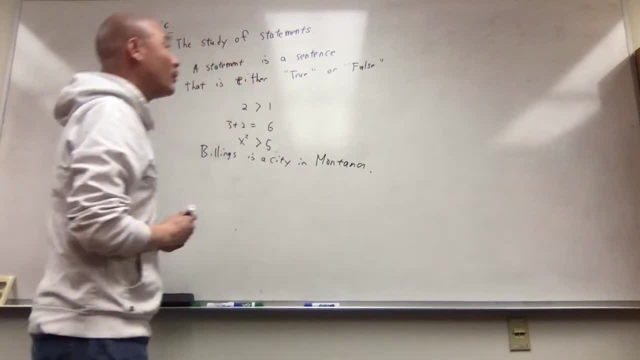 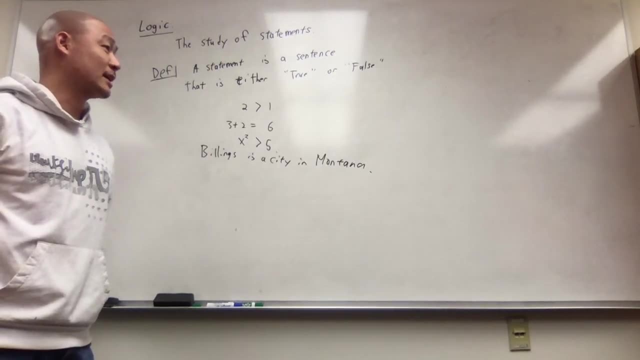 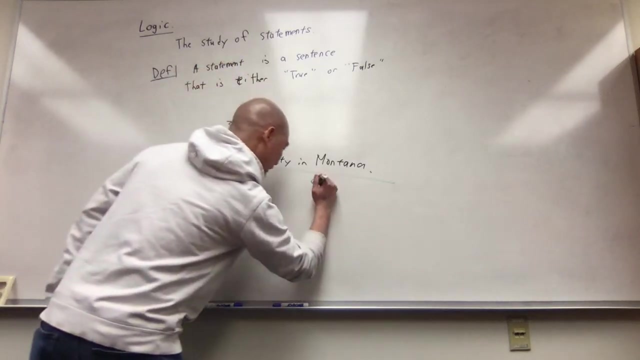 the value of either true or false. now, what we're going to do in this section, of course, is we're going to be studying statements, operations on statements and compositions of statements, which are very similar to composition and operations on numbers. so let's say, as an analog: here we have numbers and here we 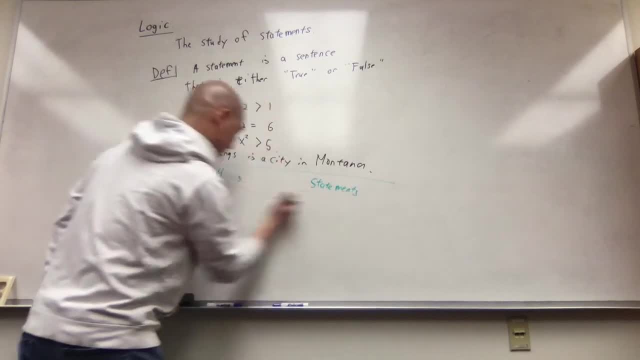 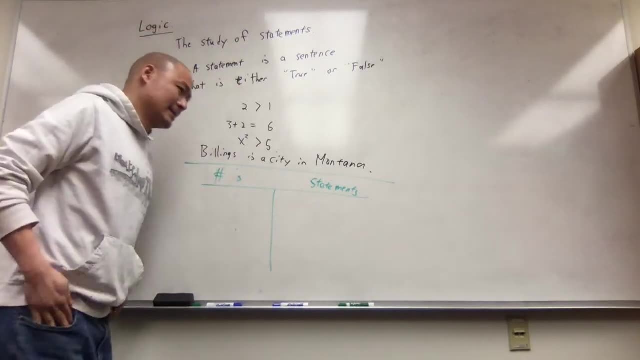 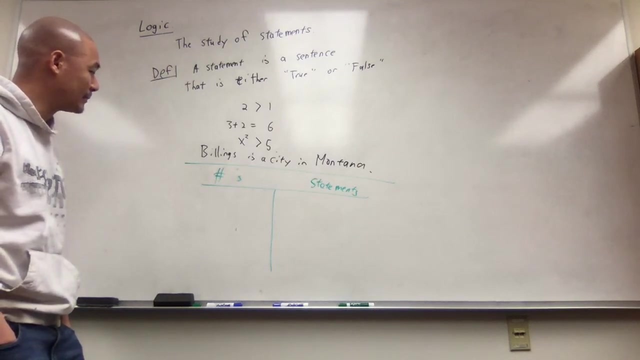 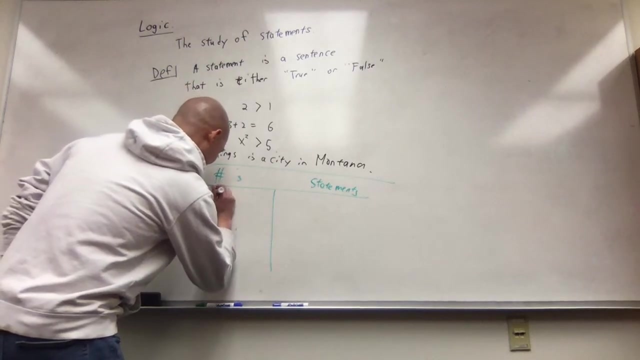 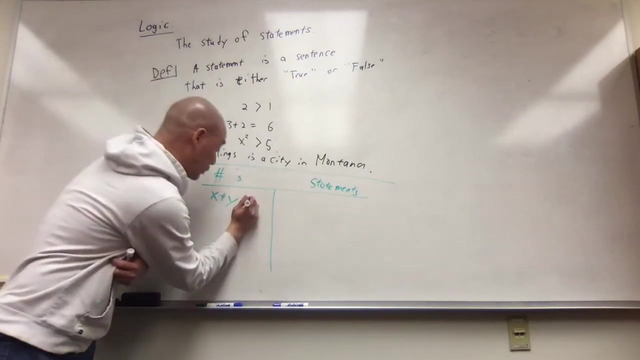 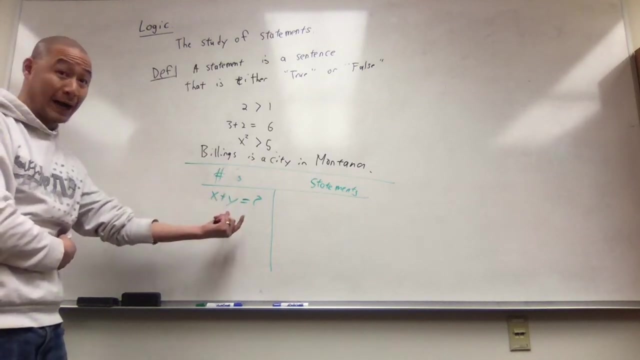 have statements. so in the typical math class you might have something like that deals with numbers like X plus Y. and what is this? equal to well, it depends on the value of X, on the value of Y, right? so X is a number, Y is a number, X plus Y is also a number. so what we mean 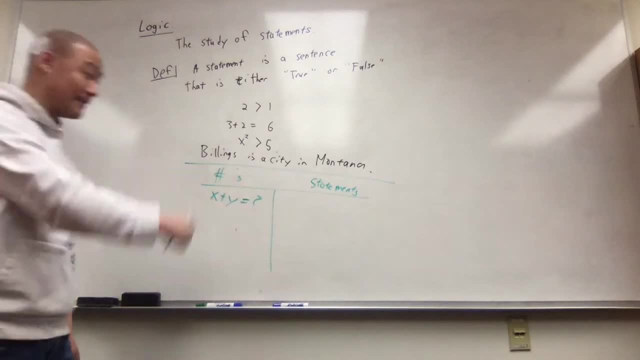 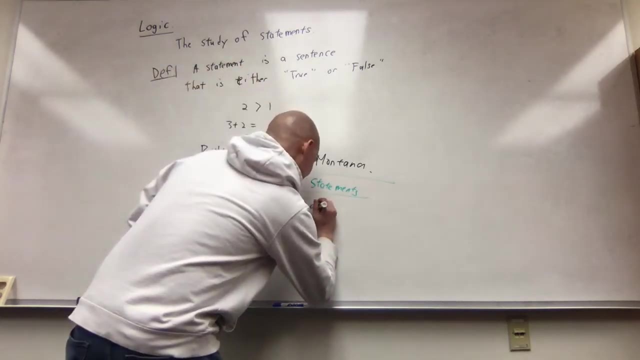 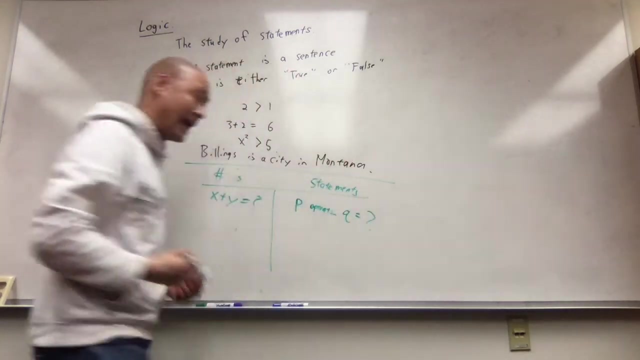 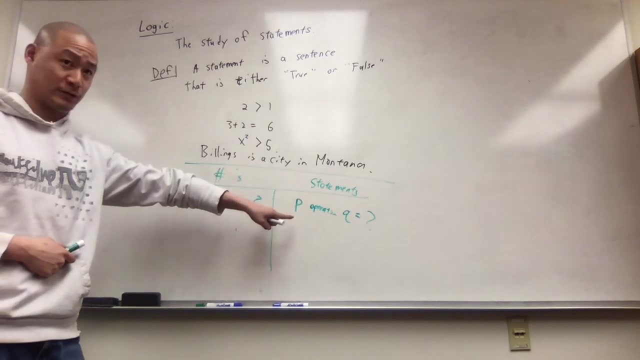 by an operational statement is would have a statement P and then some operation and then some number Q and that's gonna have some value as well. but instead of being numbers P and Q and this thing are going to take on the value true or false. right, the numbers here could have infinitely many values there's. 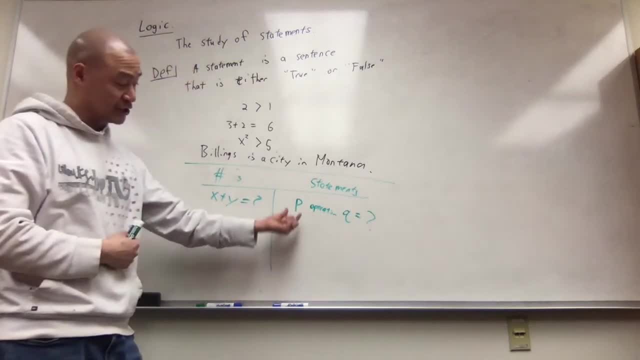 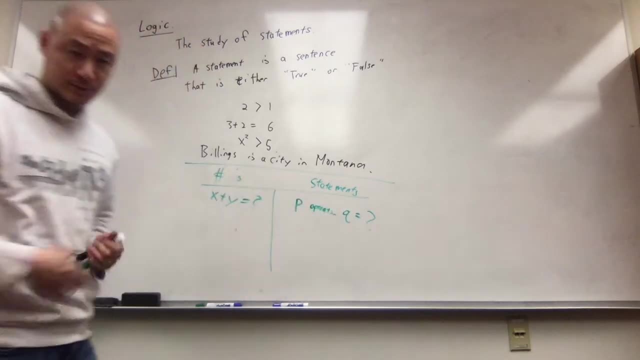 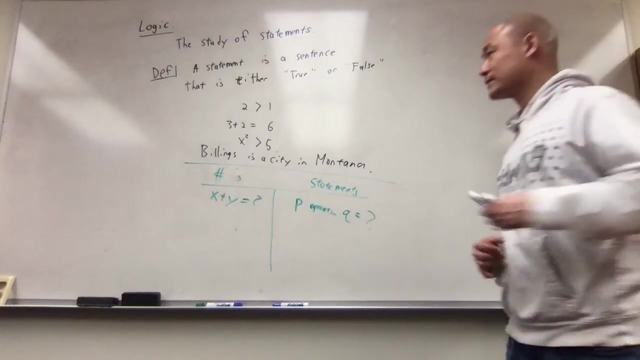 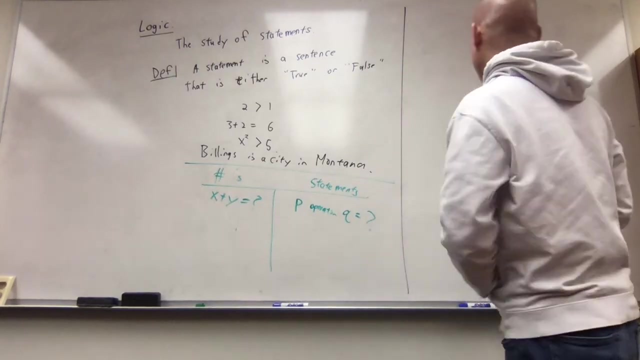 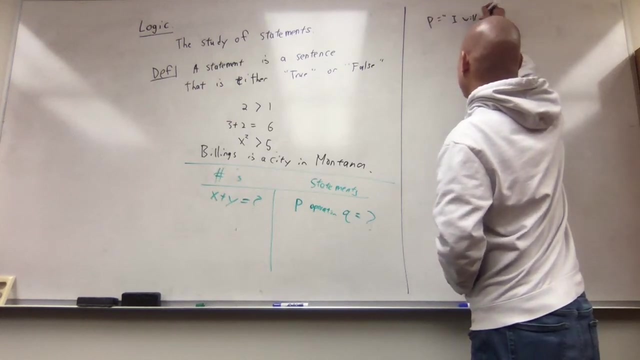 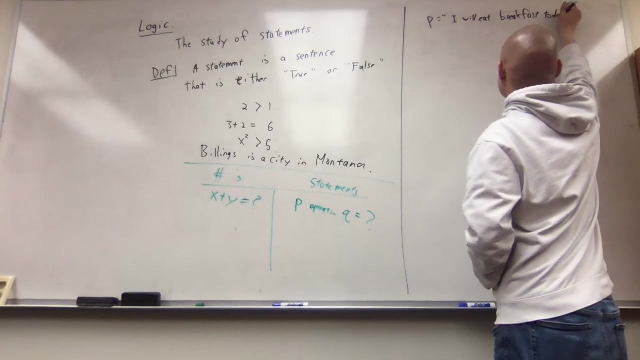 infinitely many values that could be here, but depending on operations here, P could either be true or false, Q could either be true or false, and the resulting thing is then either true or false. all right, so you, you, let's see here, let's see here. let's suppose P is the statement I will eat breakfast today. the first example of 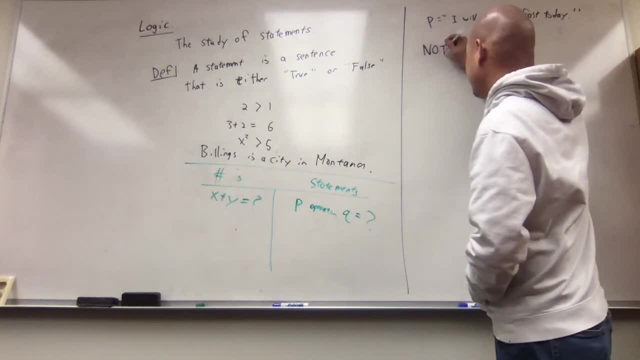 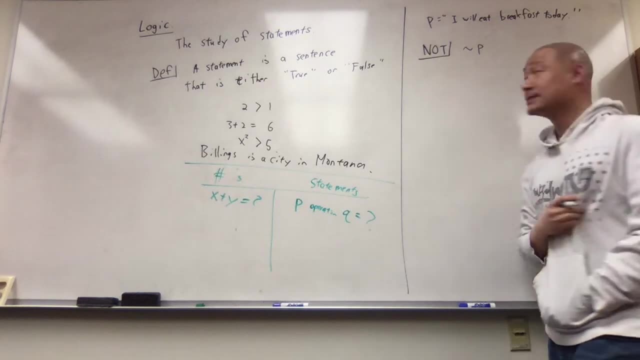 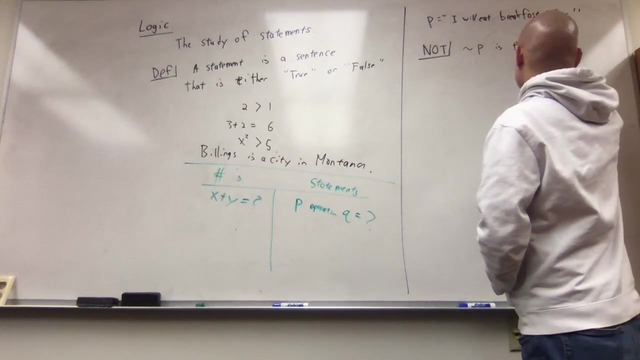 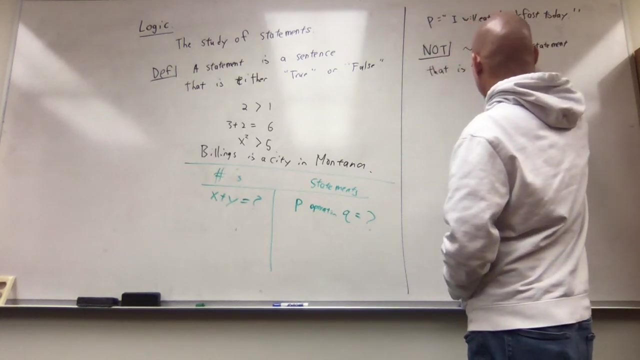 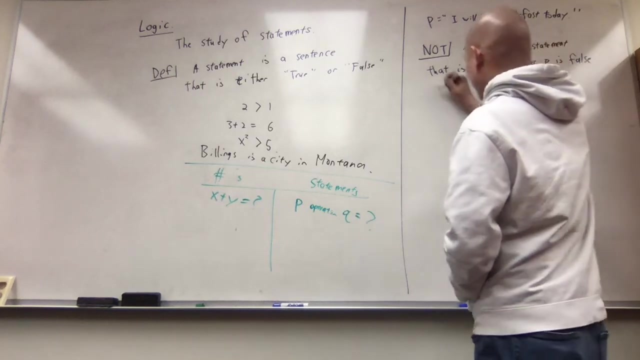 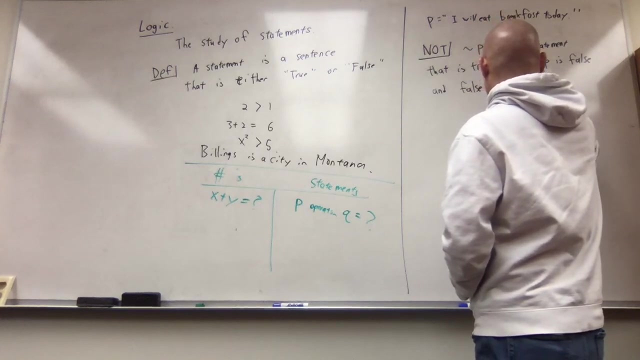 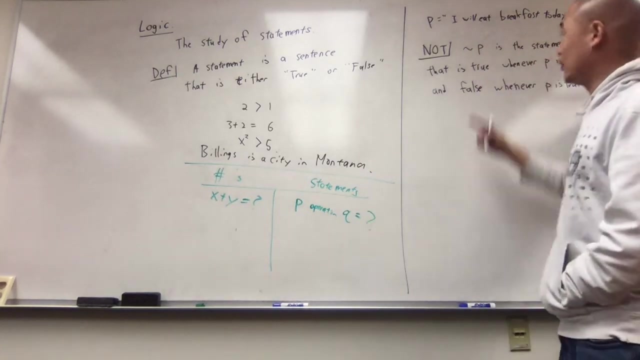 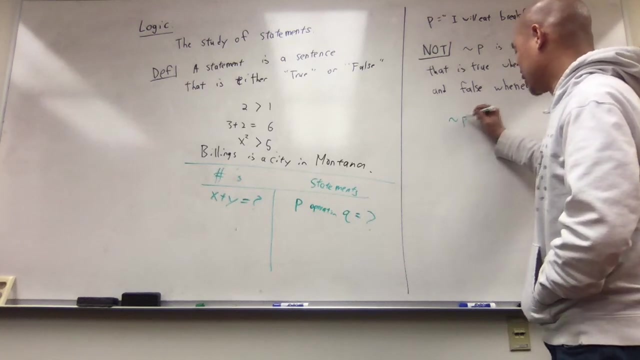 operation is the not operation, which we describe as not P. so not P is the statement that is true whenever P is false. and false, you, you, you whenever P is true. and so in our example here, if P is the statement I will eat breakfast today, then not P should naturally be what. what do you think it is? 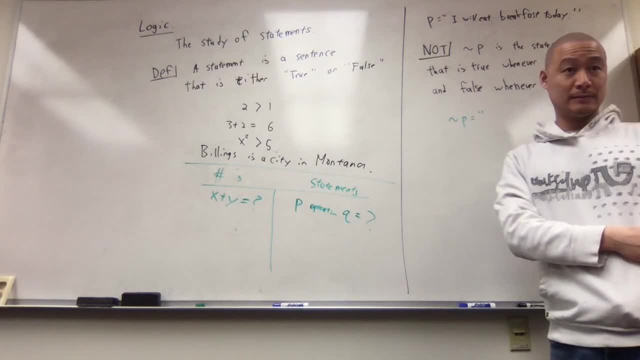 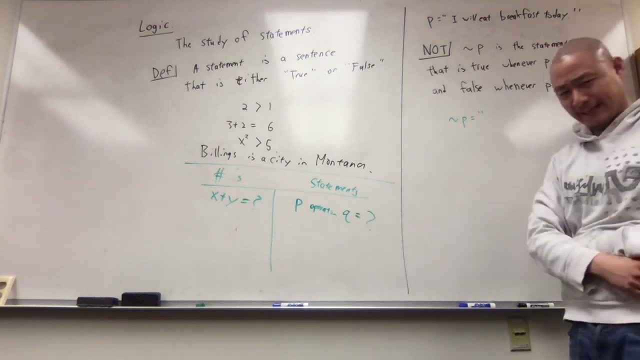 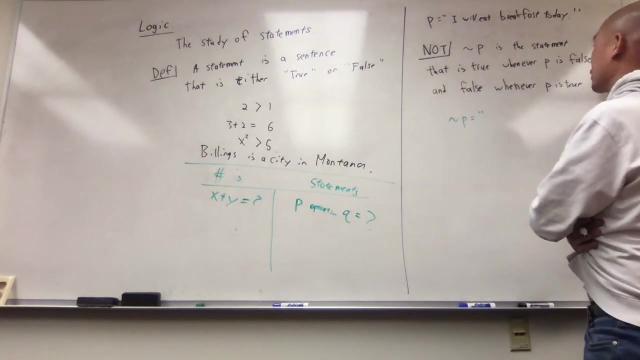 you, you, you, you, you, you, you. oh, you've been paying attention to everything I've been saying here, right? and so my stepson is behind the camera here, so right, so So P is the sentence that says you'll eat breakfast today, so what's not bad? 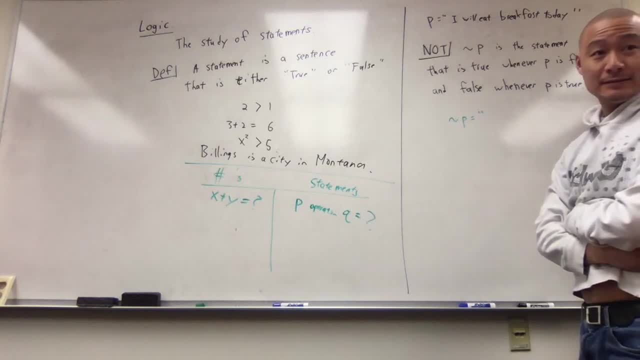 T Models. What does NOT P mean then? yes, Yeah. so what is that then? if P is eating breakfast today, then what is T NOT P? P means what's not p in Chinese: not to eat breakfast today, then what is P not in Japanese: not to eat breakfast. 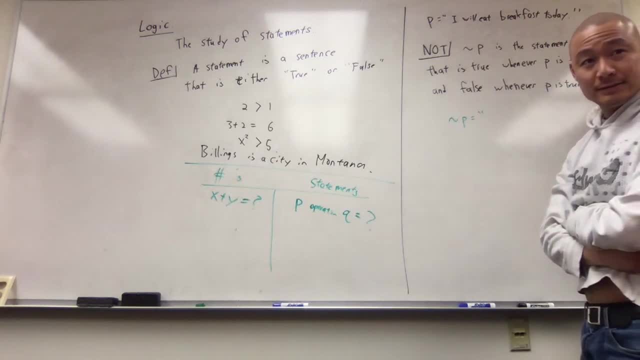 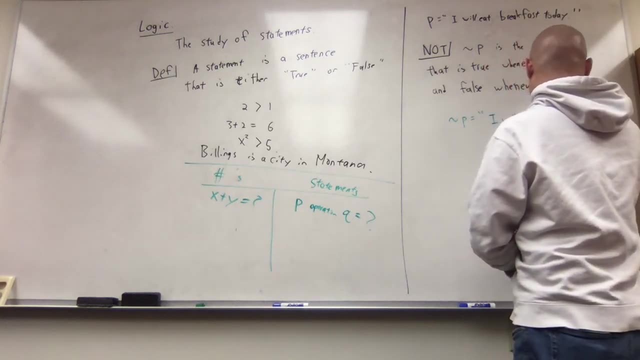 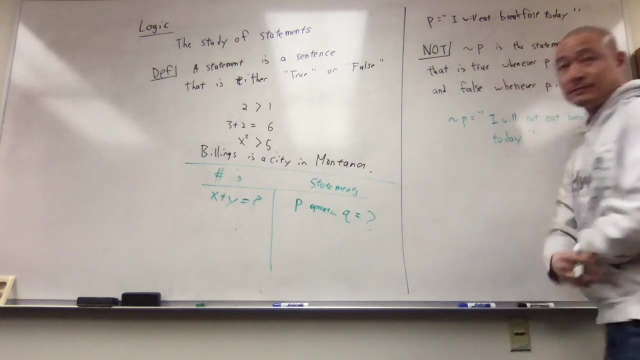 not happening exactly. i will not eat breakfast today, okay, if you're just looking for a statement that's true whenever p is false and false whenever p is true. so if p is a statement that's true when you eat breakfast, then the negation or the knot of that statement is a statement that's exactly the opposite of that. so not eating. 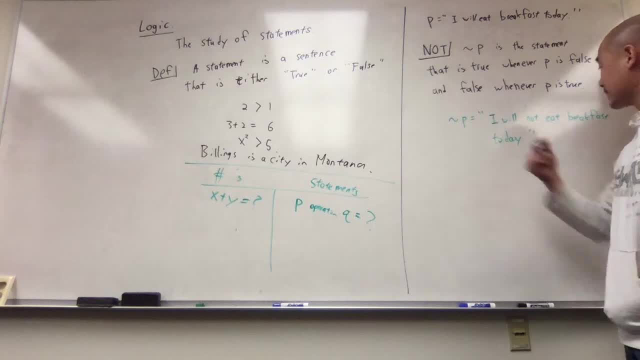 breakfast today. if you eat breakfast, then p is true and not p is false. if you don't eat breakfast, then p is false but not p is true. so that's exactly the circumstances that determine that and what we would describe as a sort of table to sort of illustrate that is. 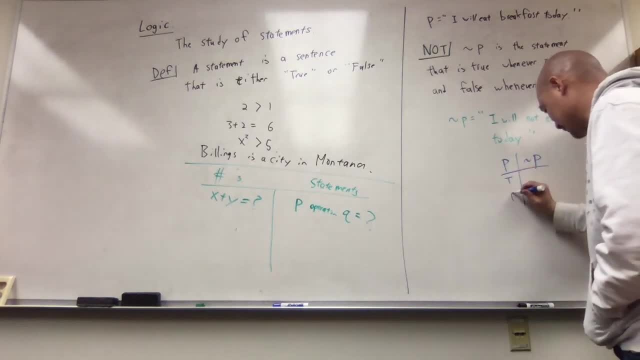 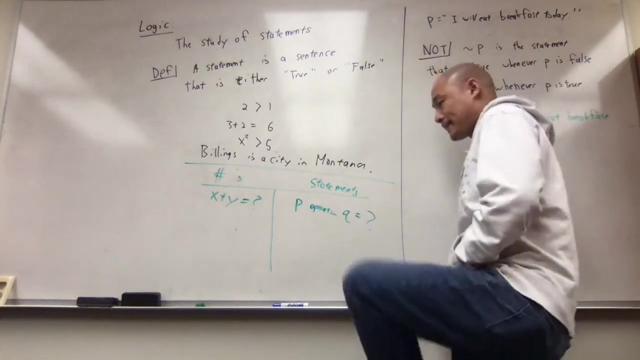 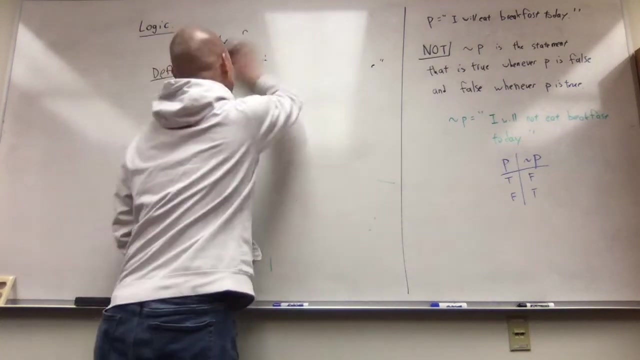 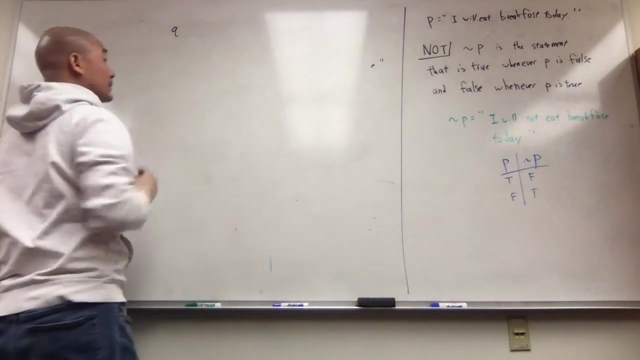 something called a truth table. so what we would say here is: for both values of p, that is either true or false. the not p's values have to be false or true. all right, I'm gonna add a second operation to this whole mess, or second statement, sorry, we're gonna add one more or two more operations, but Q I'll add to. 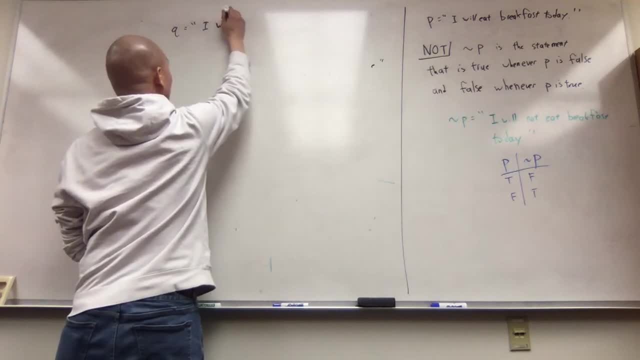 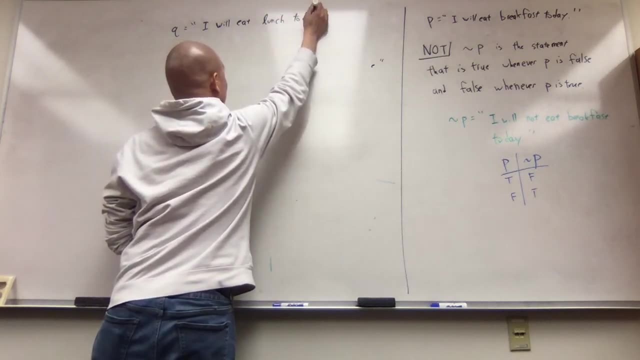 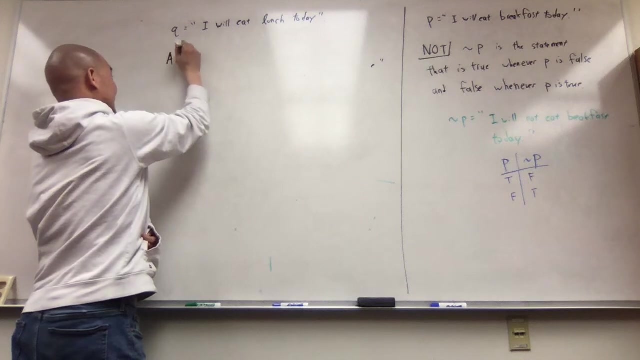 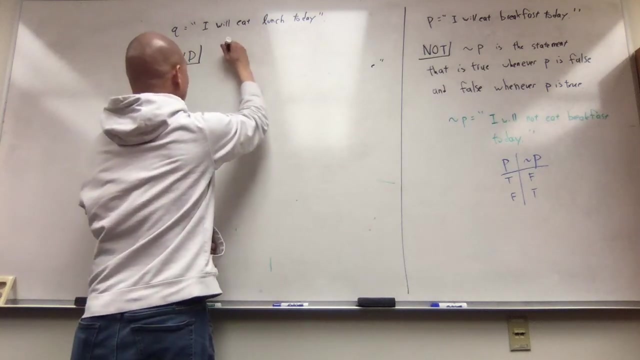 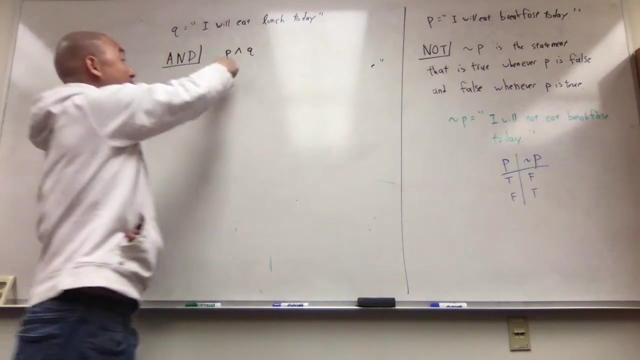 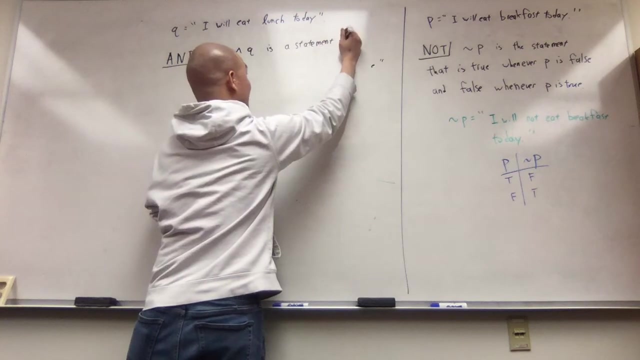 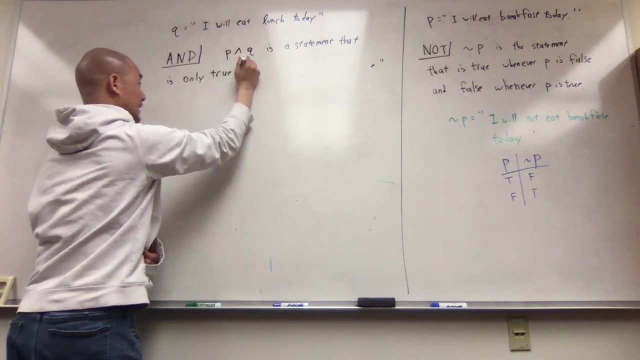 this is: I will eat lunch today and now. the second operation added in is the operation and now, and there's a statement we express, and as with this caret symbol here I would say P and Q is a statement that that is only true if both p and q. 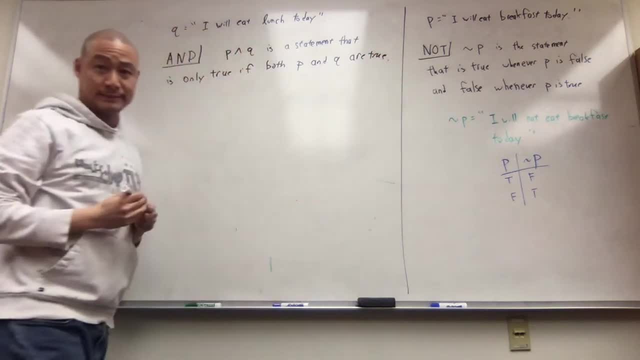 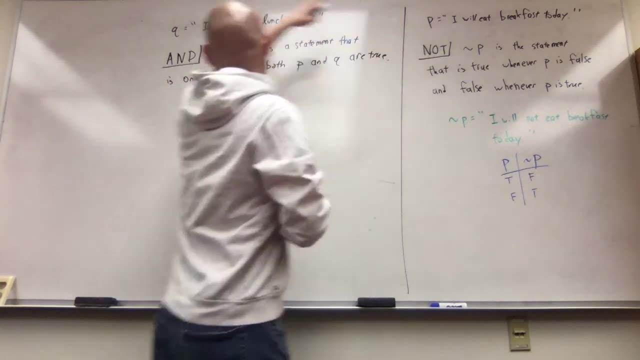 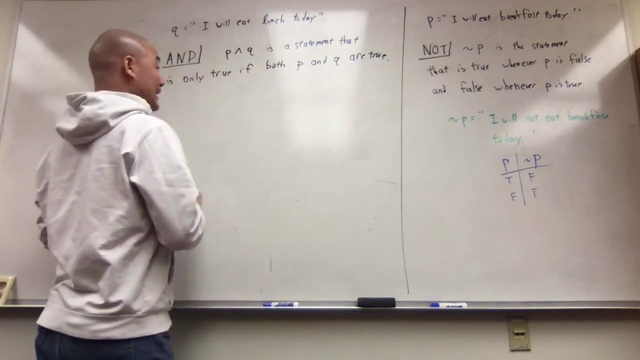 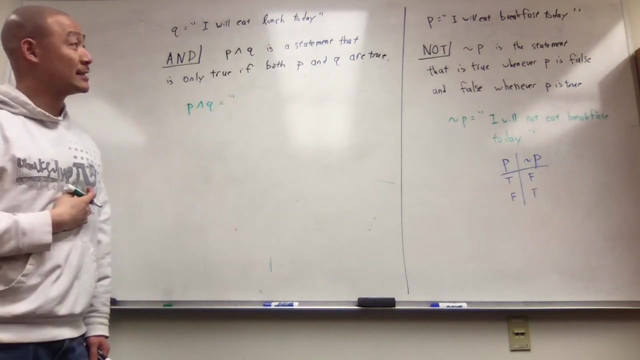 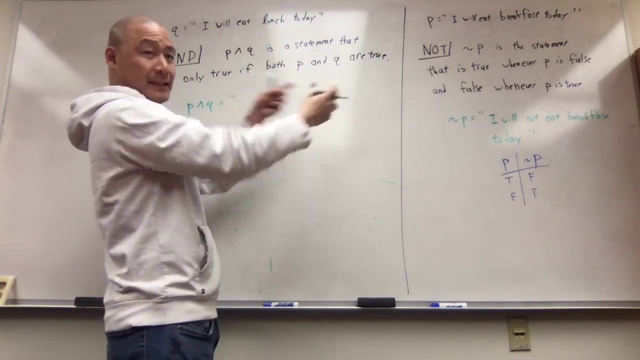 are true, all right. so so, Byron, if p is i will eat breakfast today and q is i will eat lunch today, then what would p and q be? uh, i will eat breakfast today and i will eat lunch today, if that's so, so just right. so, so it's just a statement, right? yeah, you don't need to include the. 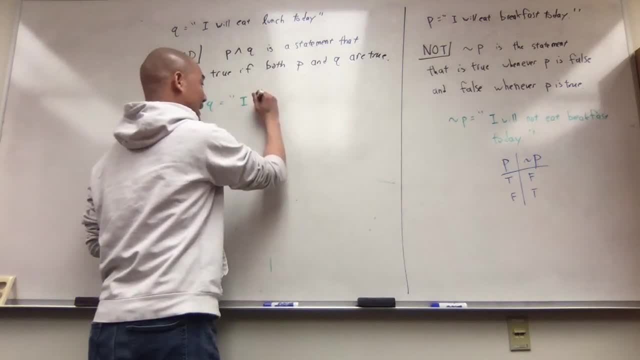 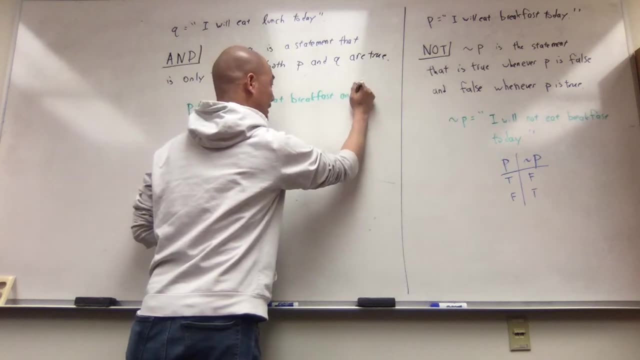 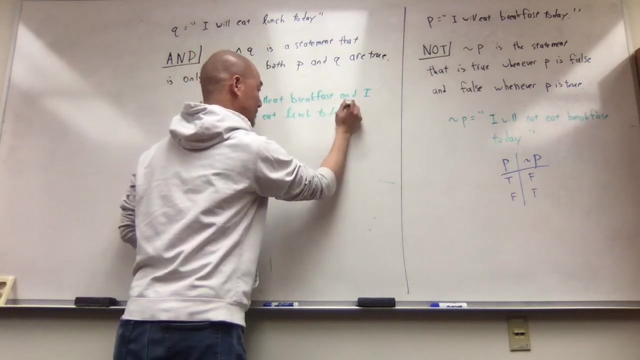 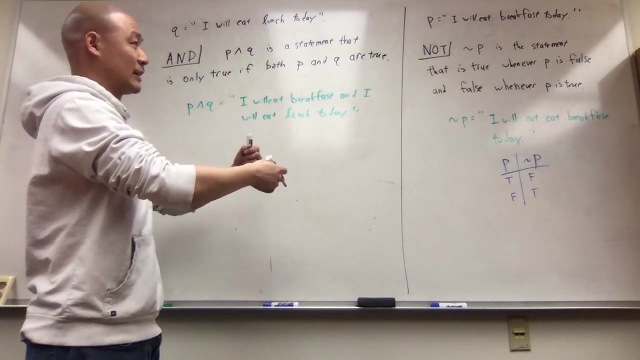 description as part of the statement. so it really is. i will eat breakfast and i will eat lunch. today there's a lot of ways you can phrase the same statement in the same way that in algebra there's a lot of ways you can uh express the same thing, right? so like: 2 times x plus 3 is 2x plus 6. 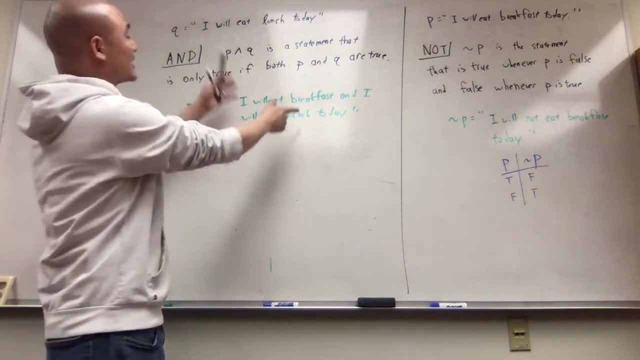 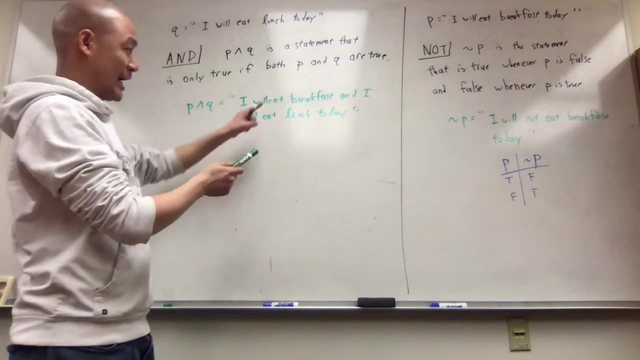 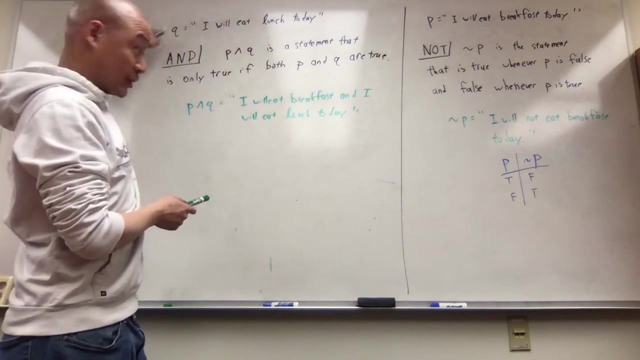 for example. and so we're not. when we make these compound sentences, we're not so concerned about the exact wording as we are, as just expressed in a statement, that is true only if p and q are true. so let's say, you do say this sentence. you say: i will eat breakfast and i will eat lunch today. 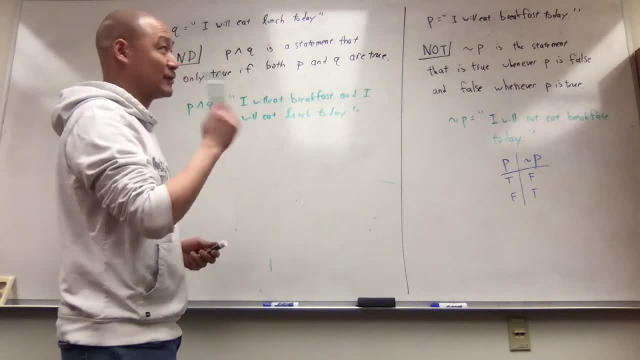 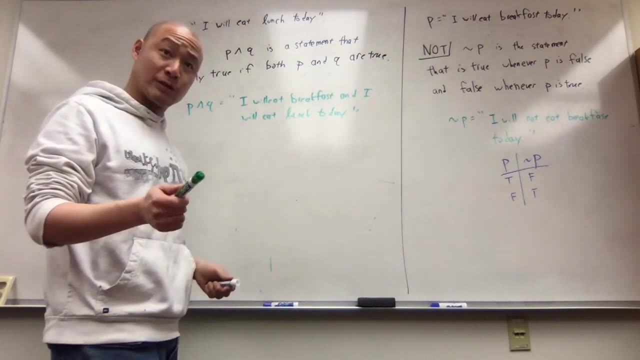 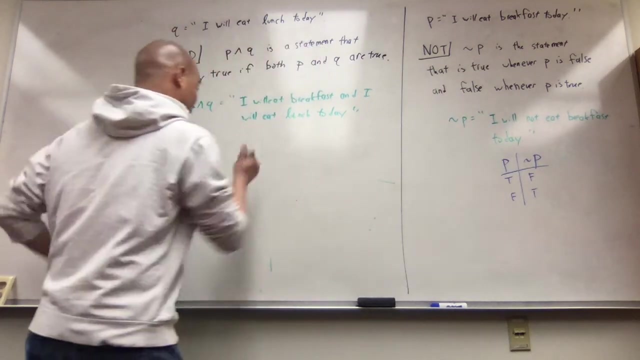 well, that's only true if you eat both breakfast and lunch. if you decide to skip one of these, then you're not telling the truth anymore. if you skip both, you're definitely not telling the truth anymore. so the truth table for something like this is a little more complex. 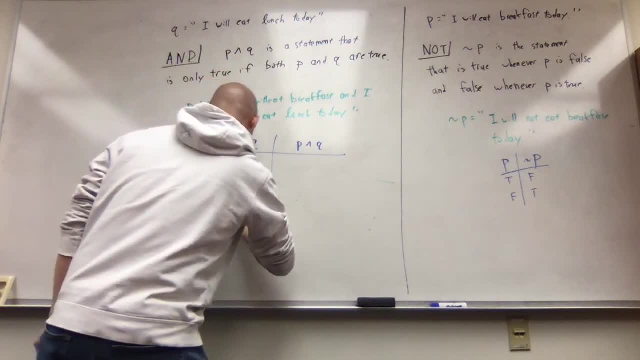 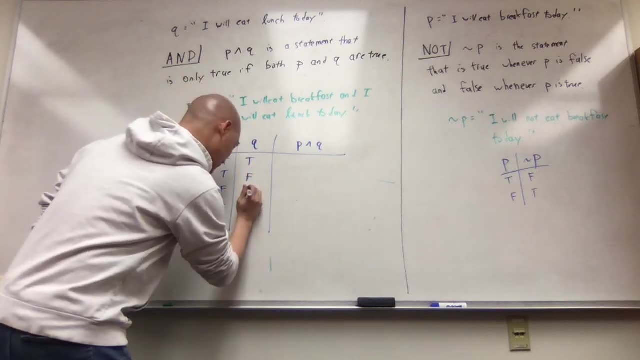 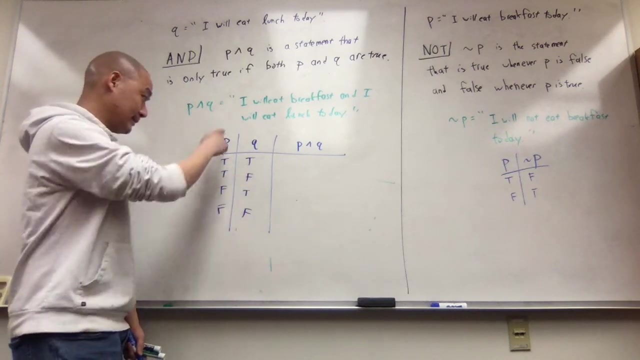 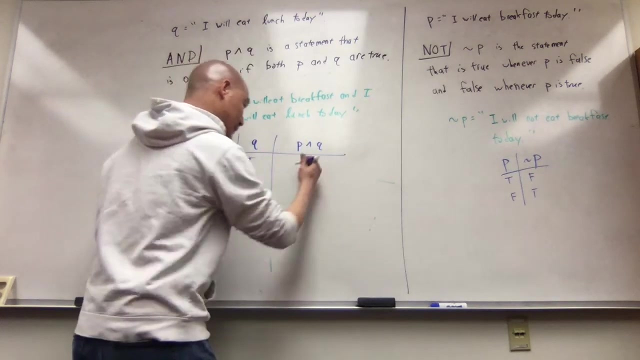 because there are two values for p and two values for q. there's four combinations in total. They are both true, P is true and Q is false. P is false and Q is true. They're both false And in this case, P and Q- it's true. 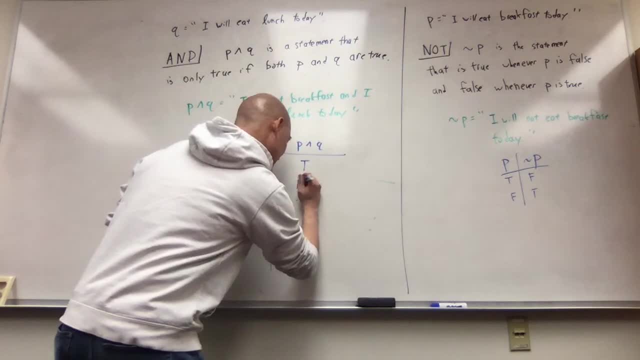 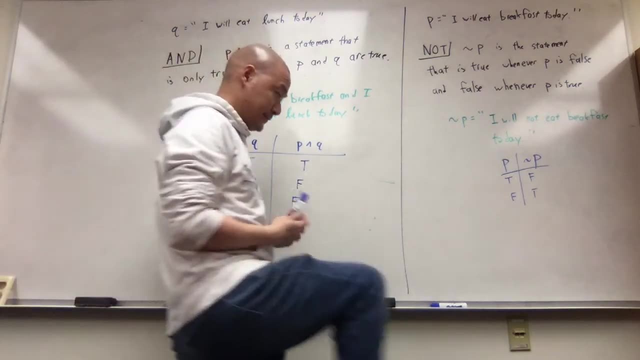 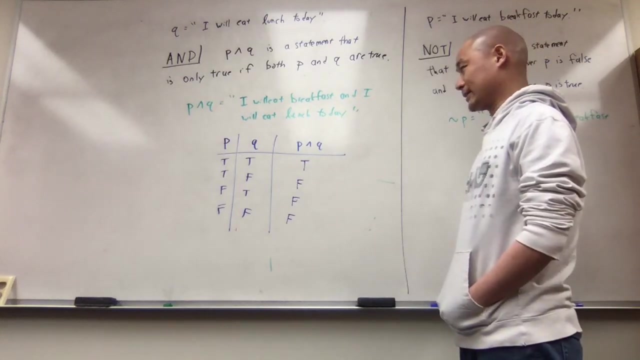 when P and Q are both true and false otherwise. And so, in the example of our lunch scenario or a meal scenario, what we'd say is: all right, if you make this statement, I'll eat breakfast and I'll eat lunch. If you end up eating both, you're. 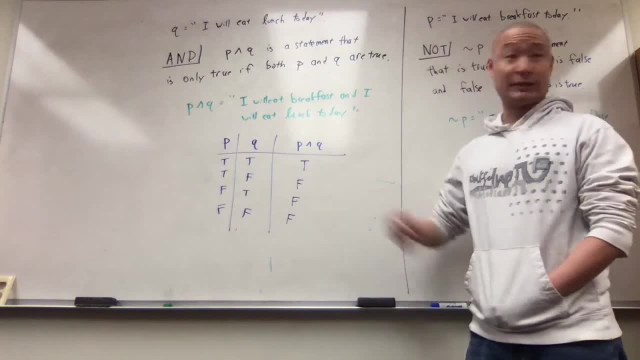 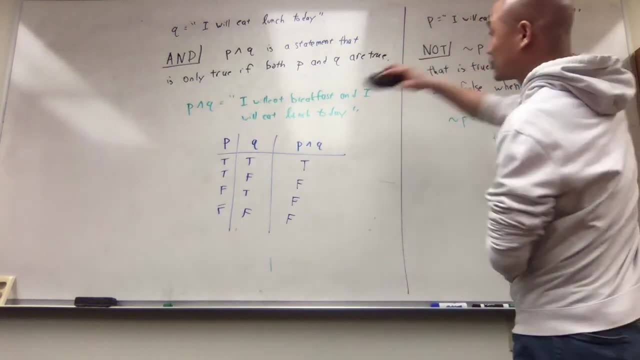 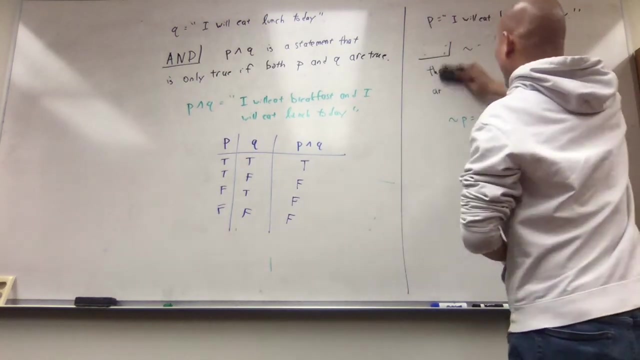 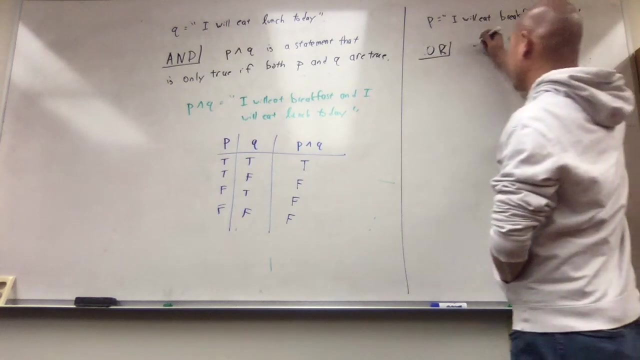 told the truth. Any other circumstances means that you lied. All right, so that statement is true if you do both false. otherwise, Then a sort of analog to: and I'm gonna keep this because we'll still use that as our example- but is or Or is a lot more forgiving than and Write or P or R. 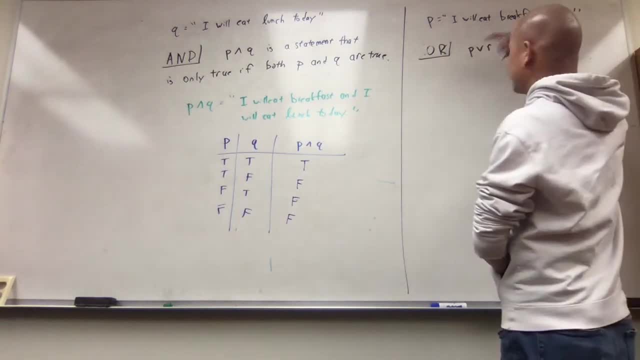 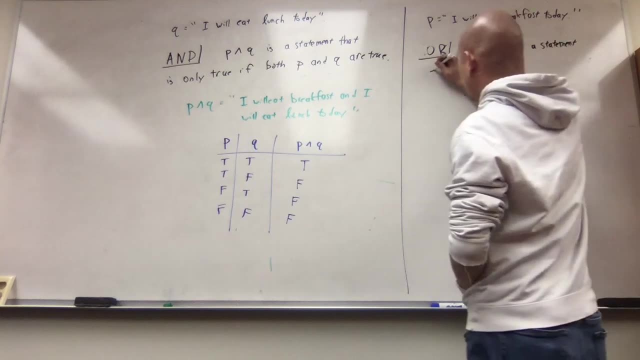 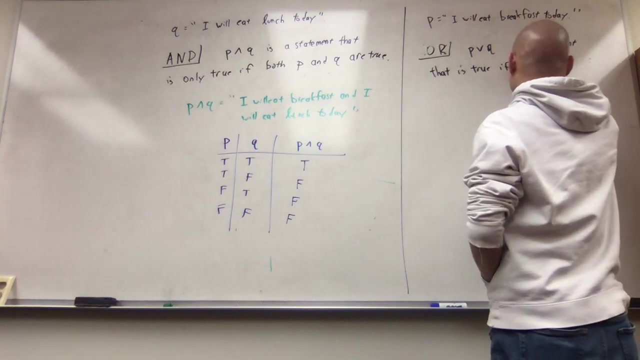 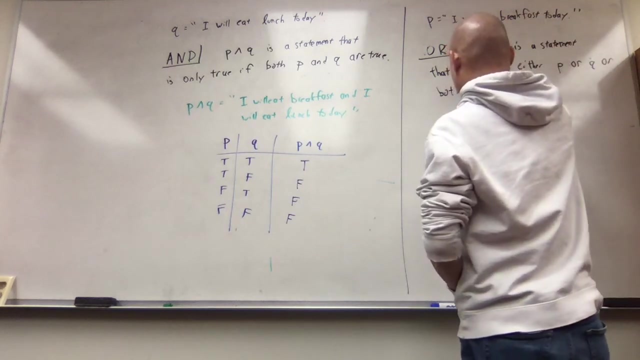 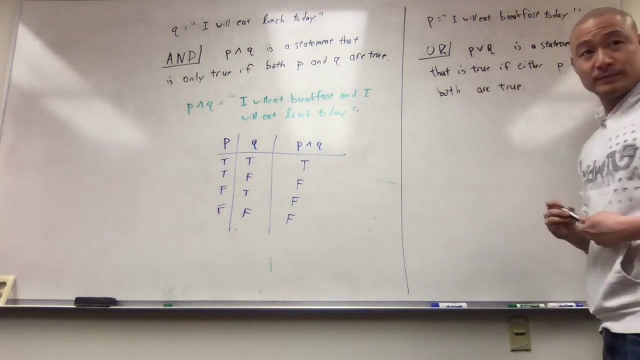 with this B like wedge here, And then we say P or R is a statement that is true, if- sorry- P or Q, if either P or Q or both are true. So if P is true, then it's true, If Q is true, then they're true, And if they're both true, it's. 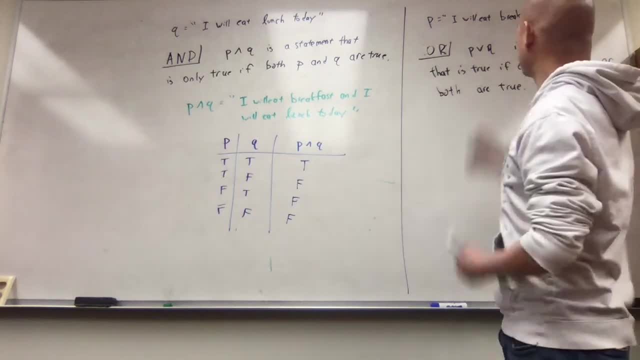 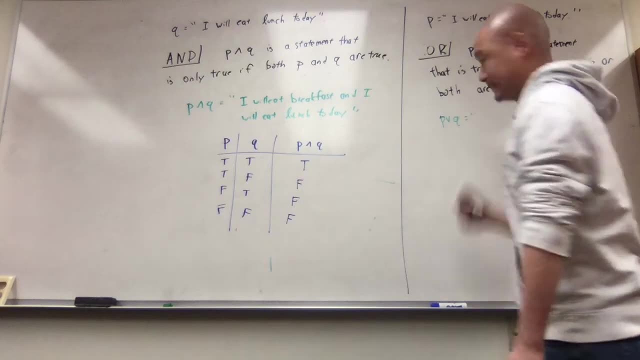 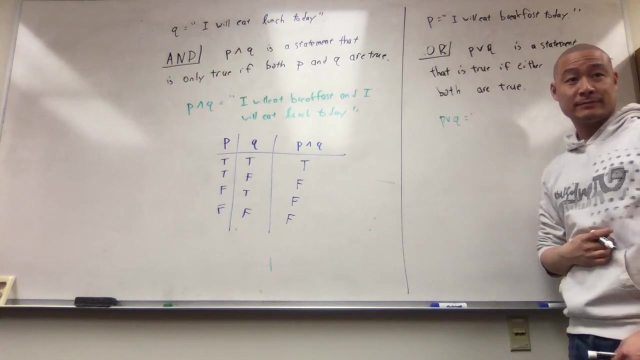 definitely true. So again, if P is, I'll eat breakfast today and Q is, I'll eat lunch. So if P is I'll eat lunch today, then P or Q. what would be a good statement? for P or Q, I will eat either breakfast or lunch today. 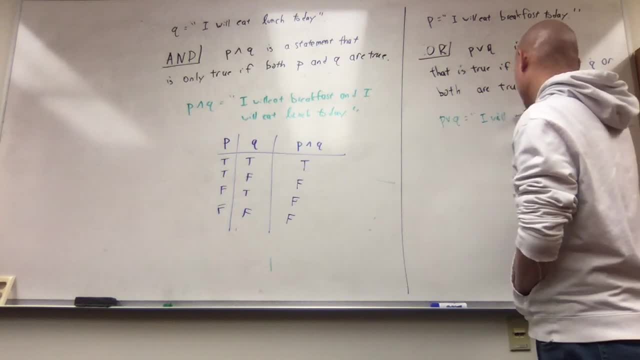 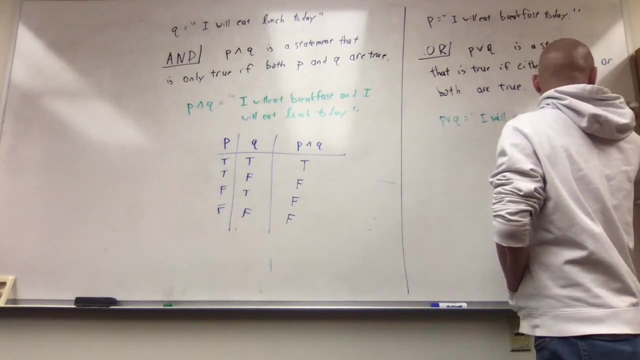 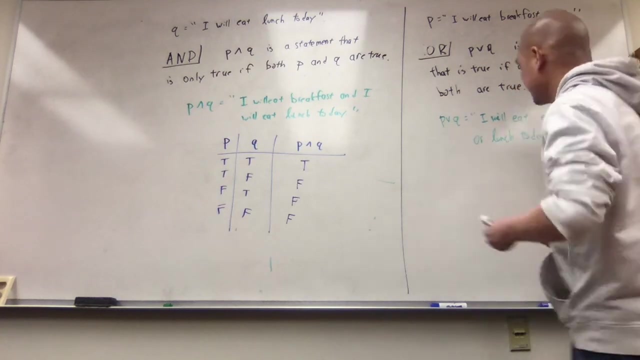 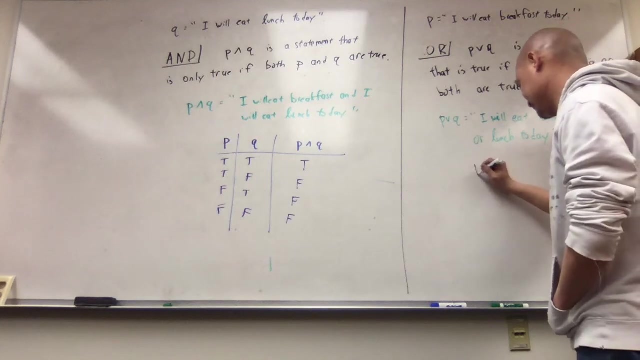 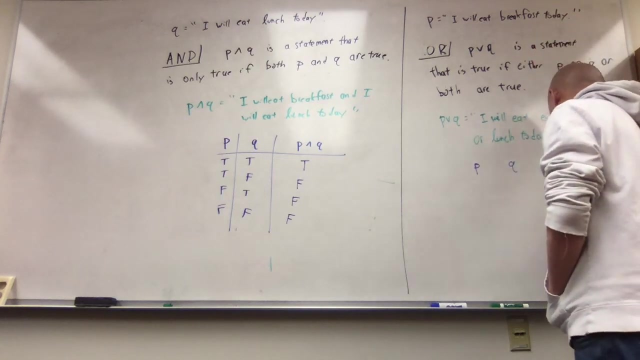 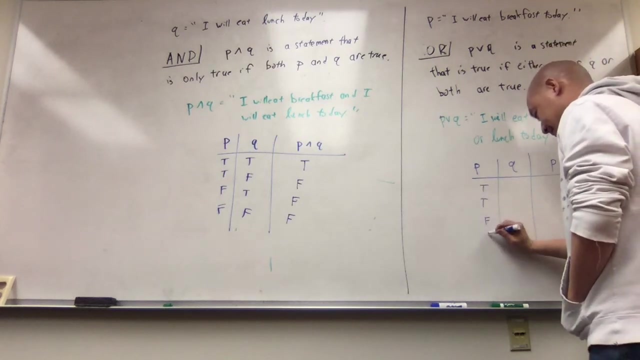 Good, I will eat. eat either breakfast or lunch today, And so let's write out the truth table for that. So P, Q, P or Q, we have our same four combinations, So I'll eat either breakfast or lunch today. 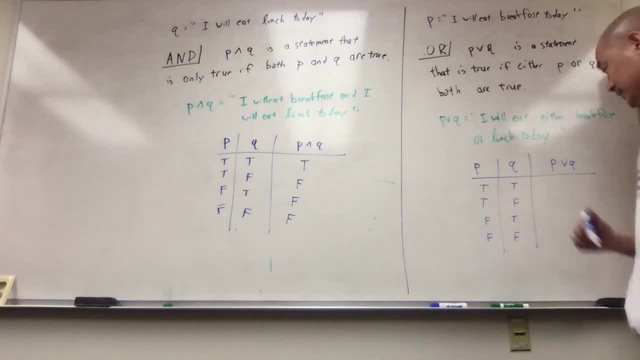 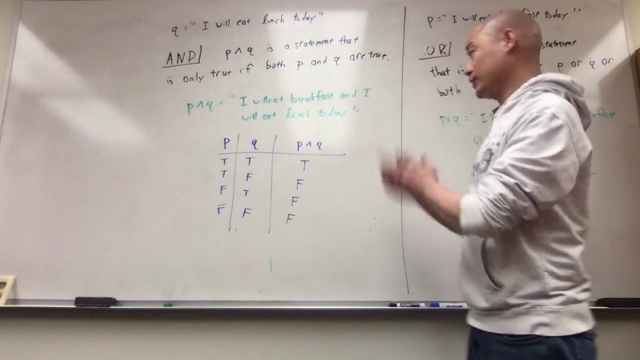 Okay, If you ate them both, is that true? True If you ate breakfast and skipped lunch, True, Is that true? Yep, If you skipped breakfast but ate lunch, True. If you skipped breakfast and lunch, False, False, All right. So, given the statements P and Q, we can compose them with and we can. 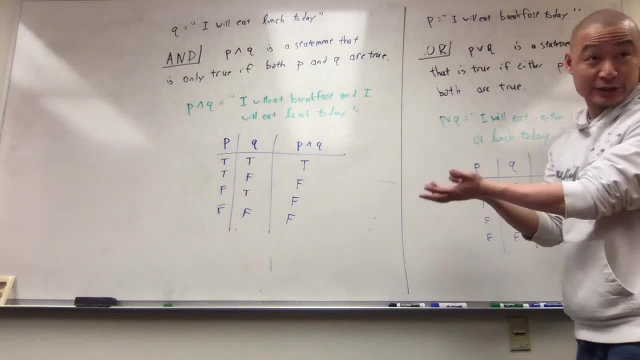 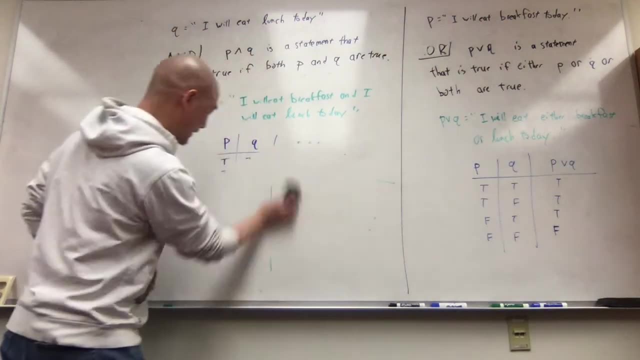 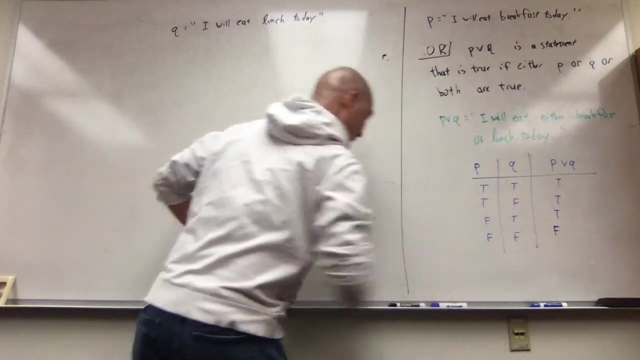 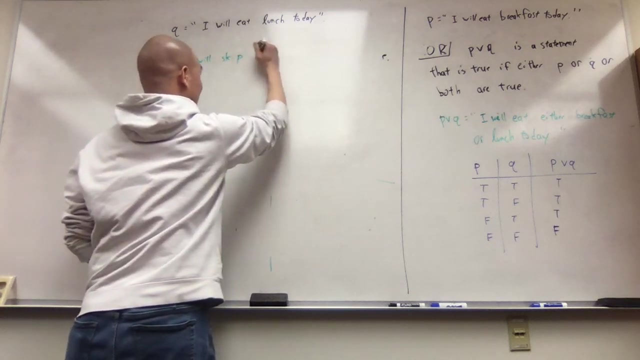 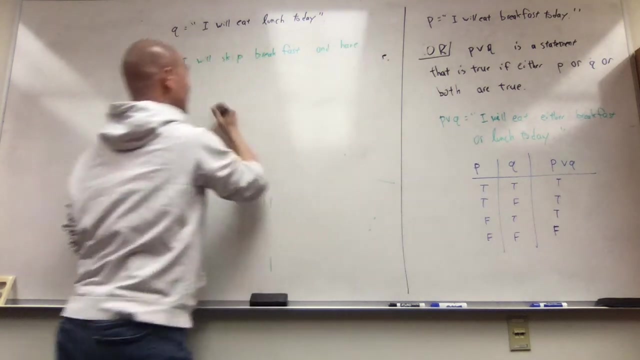 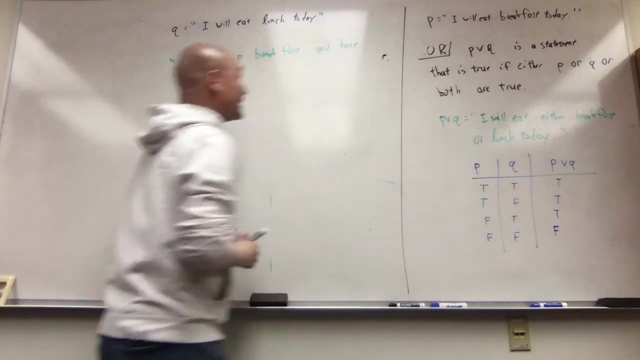 also apply nots to either statement. So let me testify in here a little with. we'll start with a statement here. Maybe I will skip breakfast And have lunch. All right, What is what would using P and Q and the operations we have described? so? 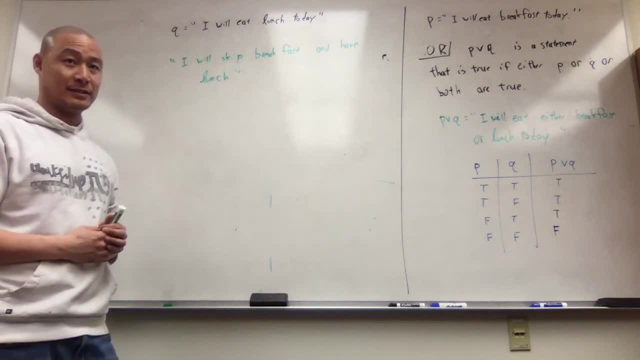 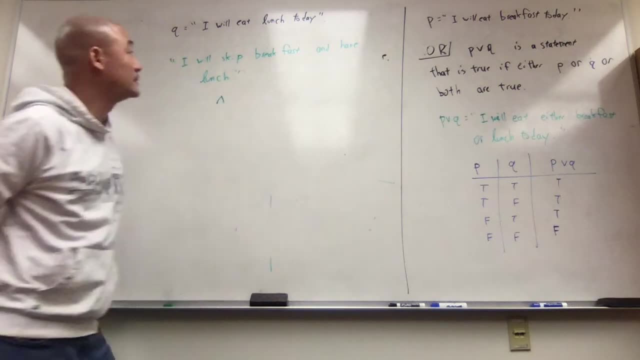 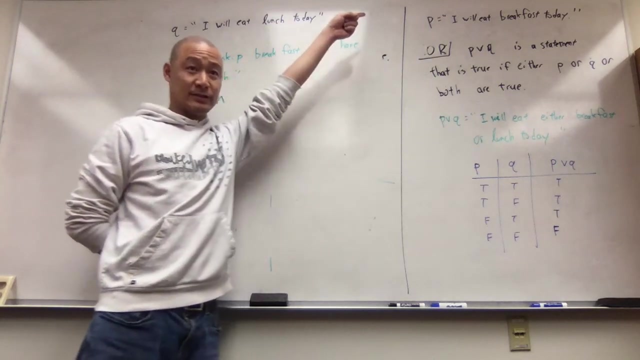 far today. what would make up this sentence here? We would definitely be using: and, of course, Okay In the sentence, Okay In there. P would be: I will skip breakfast. Well, we're stuck with these P's and Q's. 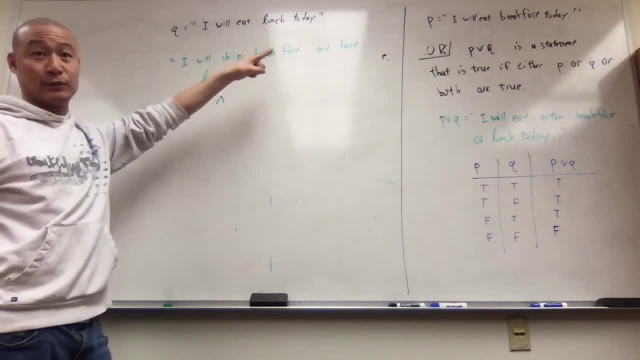 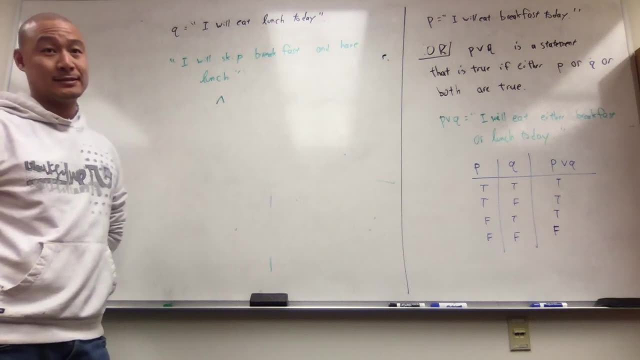 Yeah, So instead of I'll skip breakfast, what could we use Instead of re-changing P? could we express skipping breakfast in terms of P, Without changing like the wording of that? Yes, I was about to say I will not eat breakfast. 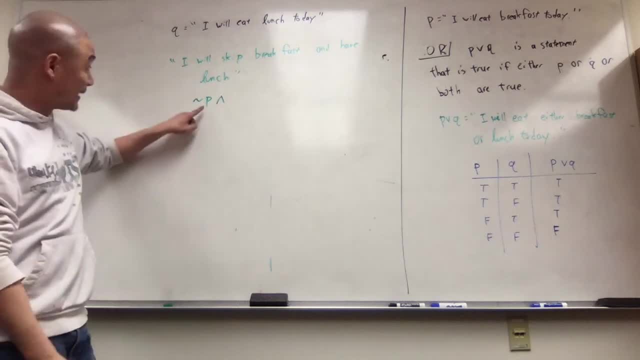 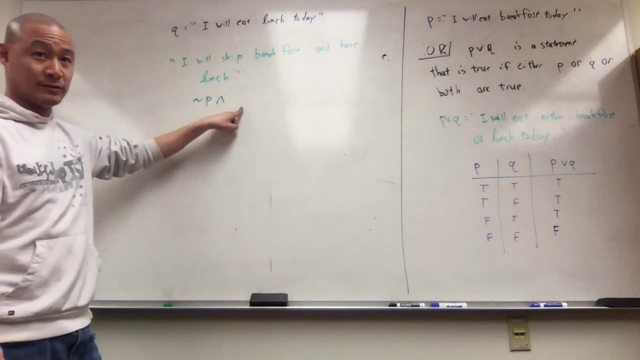 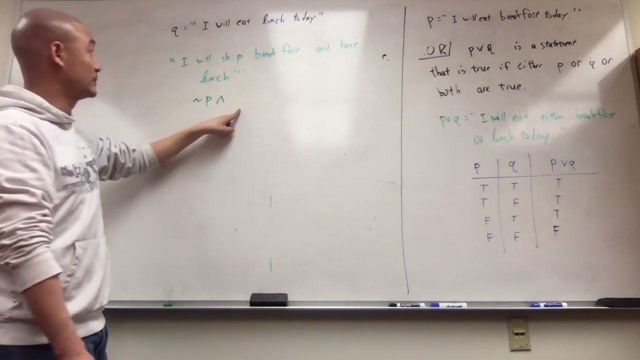 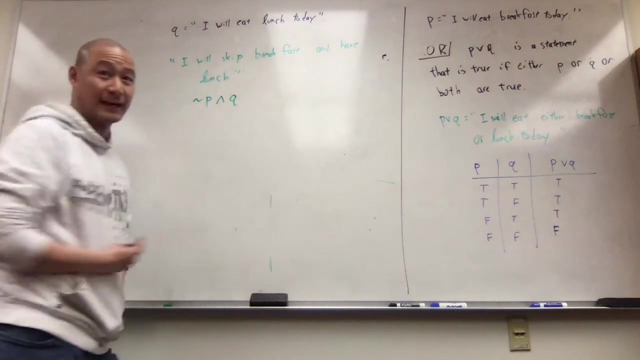 Right, P is eating breakfast, So not P is skipping breakfast. Right, And you're going to have lunch, So Right, And I will have lunch, Right, Of course. So It does seem like just Q is fine, Yeah. 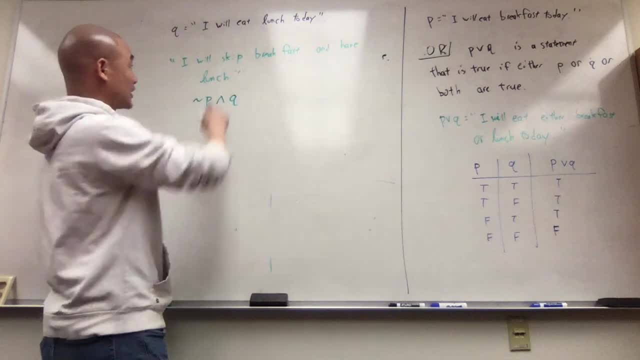 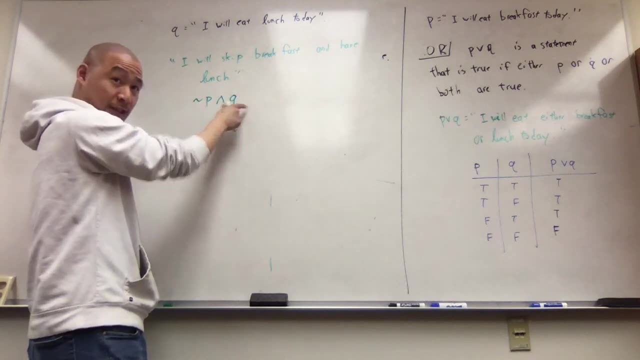 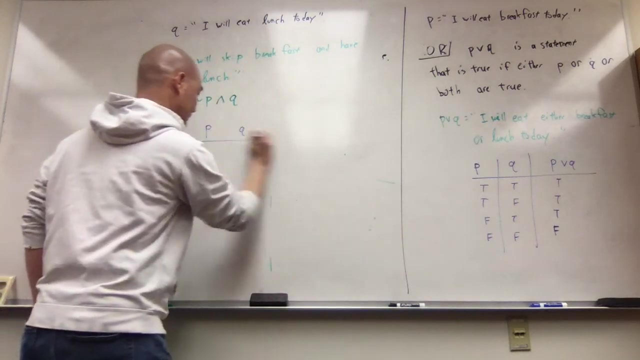 Right, So P is having breakfast, Q is having lunch, not having breakfast and having lunch. It's not P not breakfast and Q lunch. So let's see when this thing is true or false. Okay, Okay, Okay Okay. 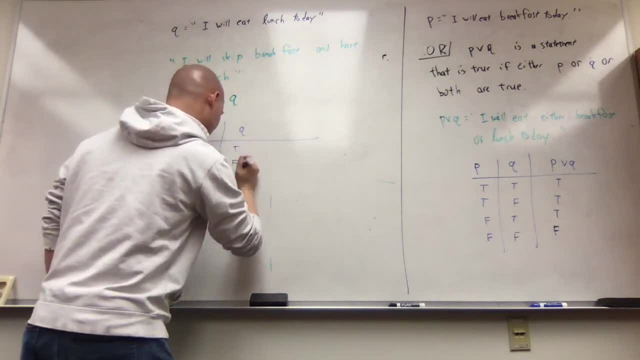 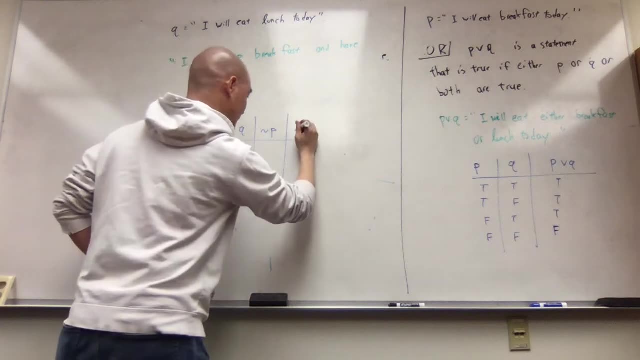 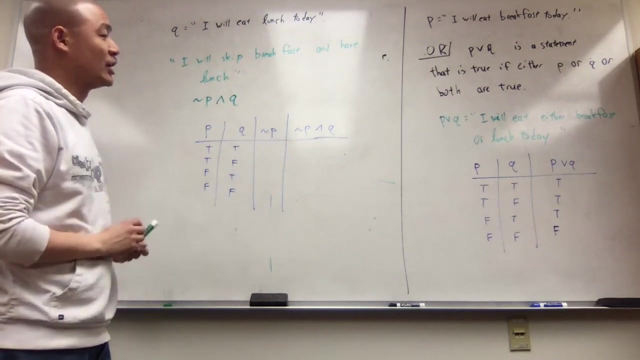 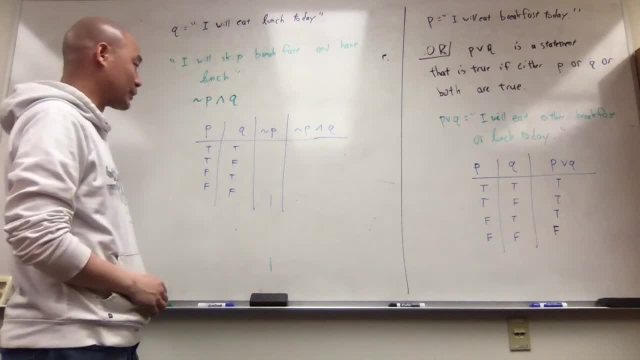 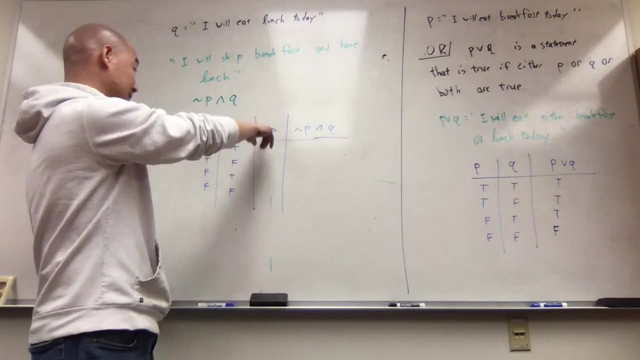 While we're still getting used to this. So here we have P and Q and other four combinations again. Alright, not P is false When P is true, So So. So I will say no A can You have togeschose with. 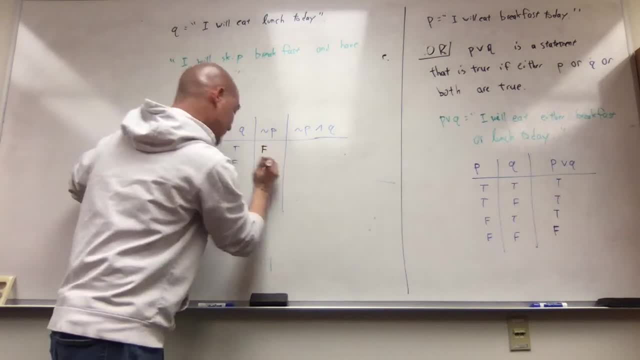 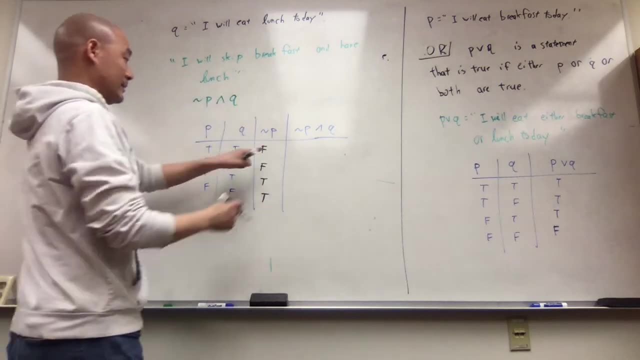 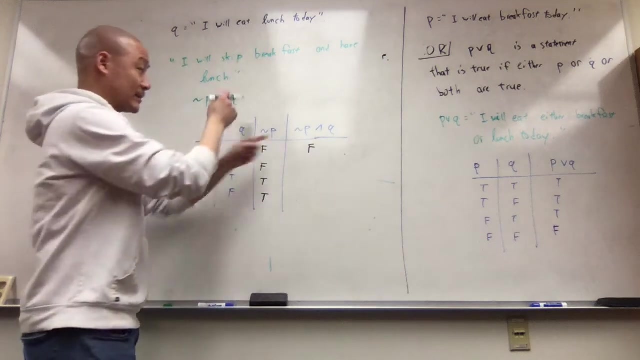 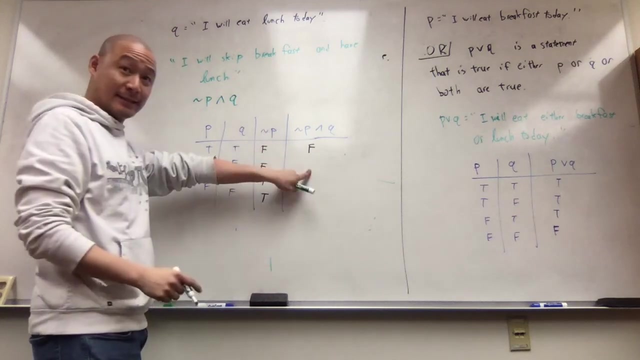 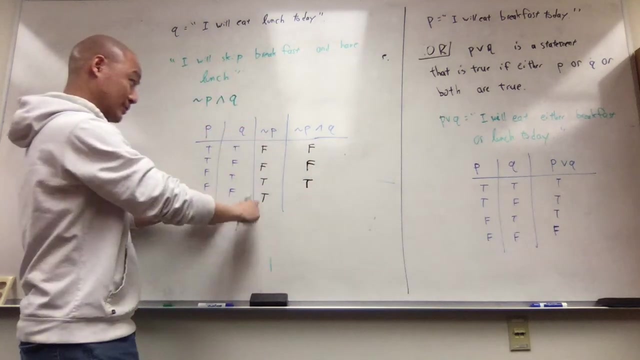 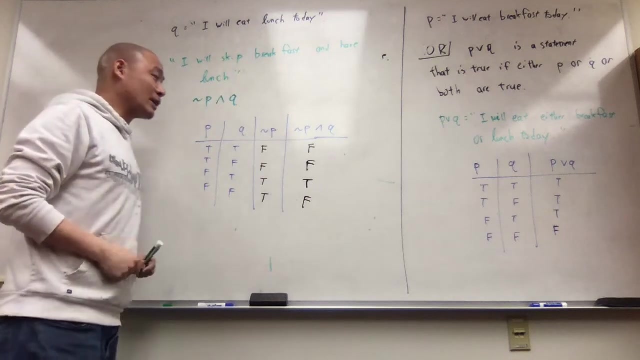 Sorry for my lunar new, I don't know. All right is true, right and it's true, and P is false. now, false and true. is folks right? that and statement is only true when both things are true. so false and false is true, and true is true and false, or true and false is false. so here we have. 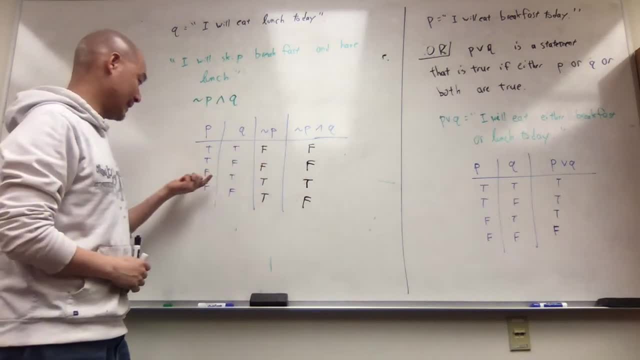 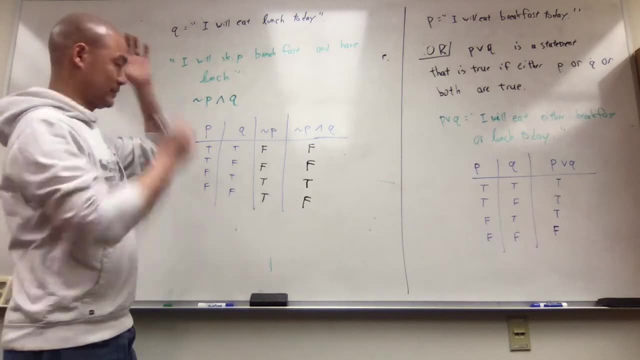 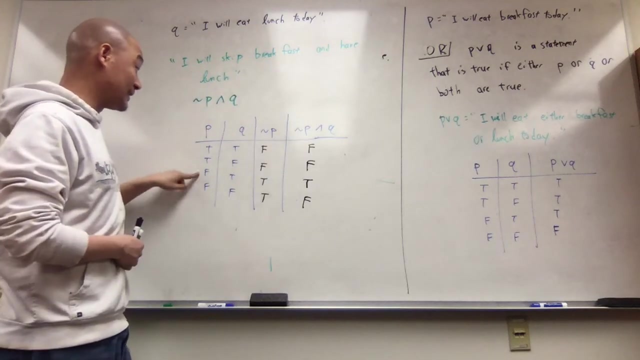 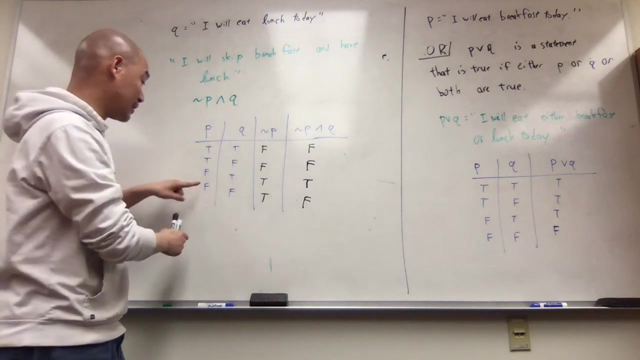 a statement that's only true in this role and false in every other role. now let's see if that makes sense, just intuitively. if you say I will skip breakfast and have lunch, you should definitely skip breakfast. you should definitely have lunch. if you don't have lunch, you're false if you eat breakfast. 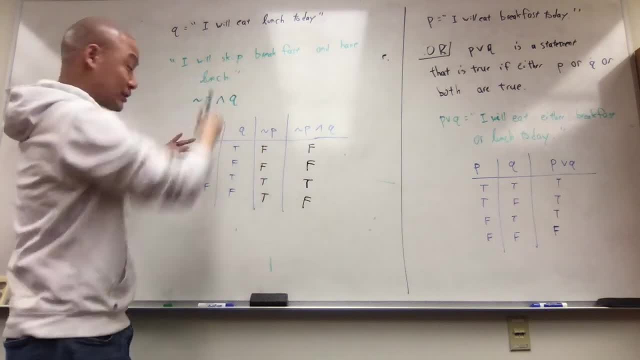 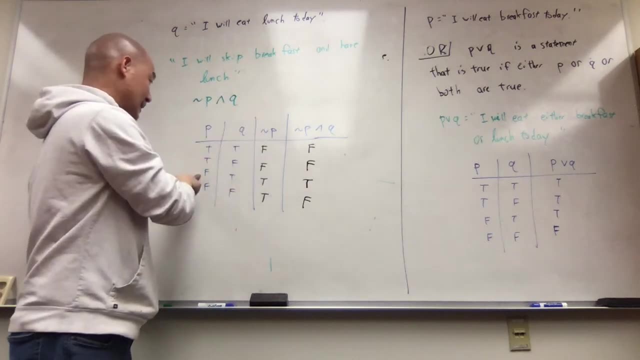 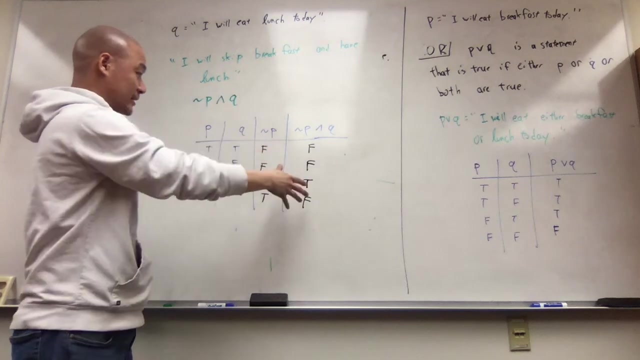 you're folks because you said you would skip breakfast. so the only circumstance under which this statement could be true is exactly when you've skipped breakfast and had lunch, like you said you would right. so when we work through the logic and when we look through this example, they should coincide. 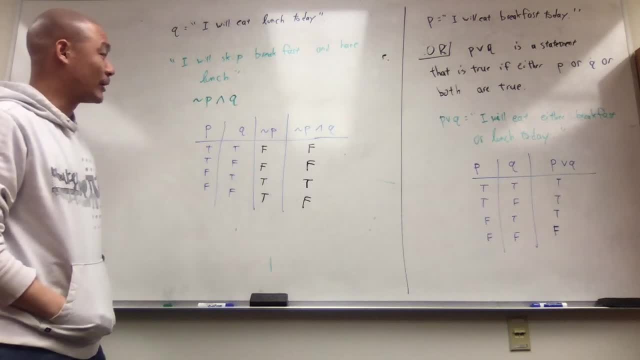 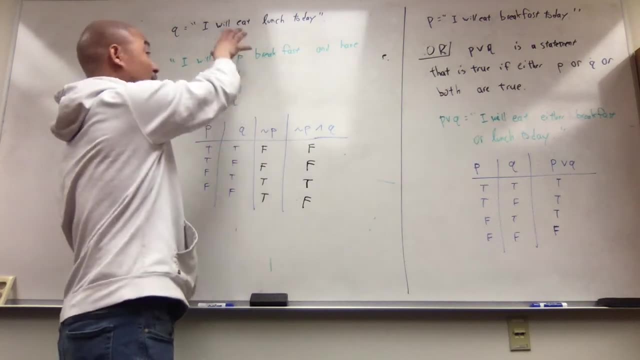 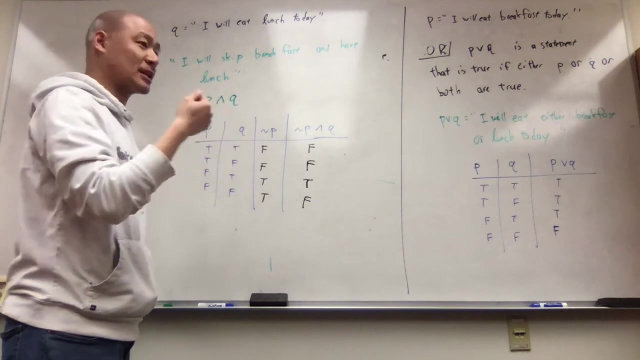 they should both make sense. now, at a certain point we will be working with just these statements, independent of some representation. in the same way, in algebra we can work with variables and numbers without having some concrete thing attached to them. but if it helps, you get used to it whenever. 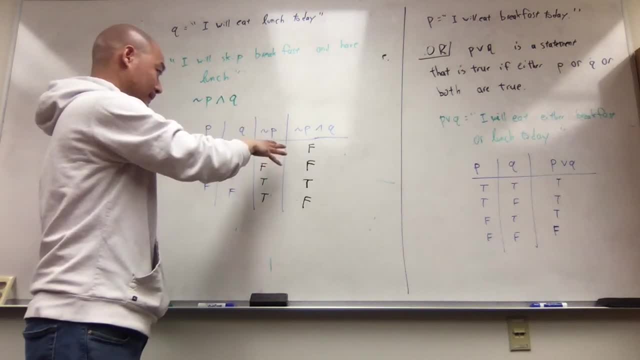 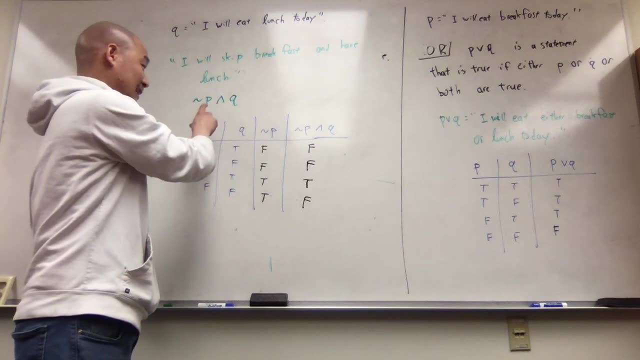 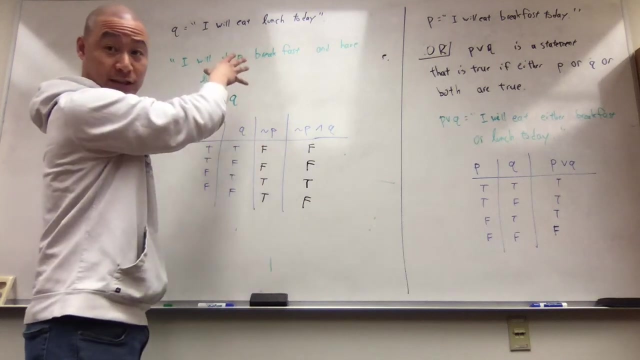 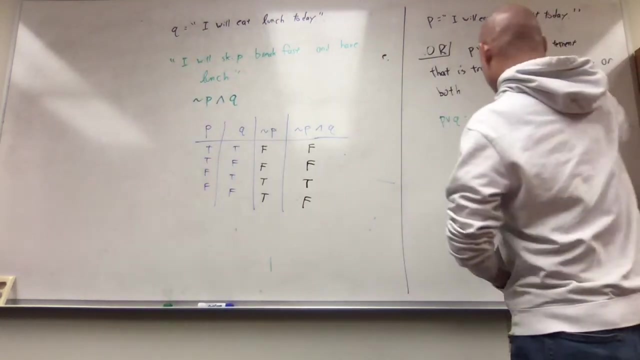 you see some collection of statements. it is certainly helpful to make up values for p and q, make up statements for these things, and then see if what you produced makes sense in relation to that. okay, then we will do one last sort of example for this video, and that is we're just going to. 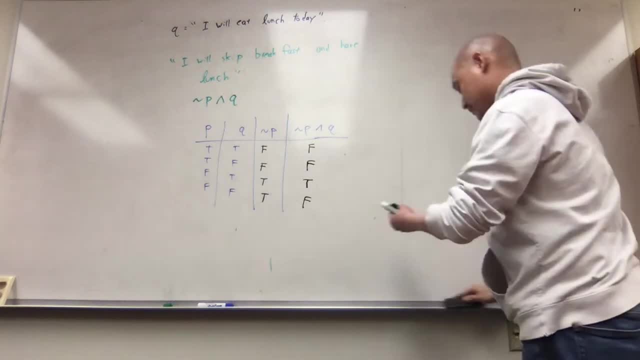 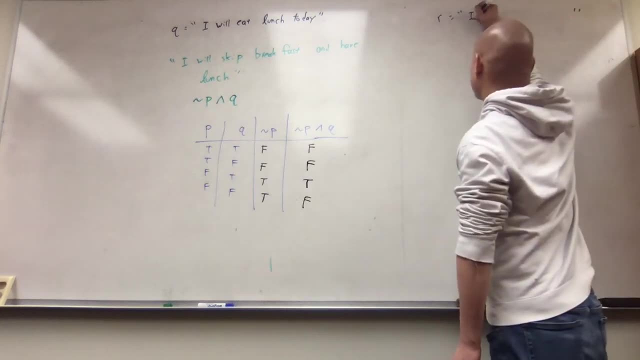 introduce you to some of the things that we've talked about in this video. and we're going to introduce you to some of the things that we've talked about in this video and we're going to introduce a third variable, r. certainly we could say that r is i will eat dinner, or something like. 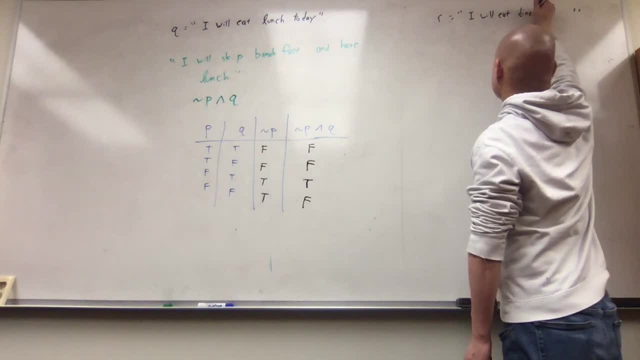 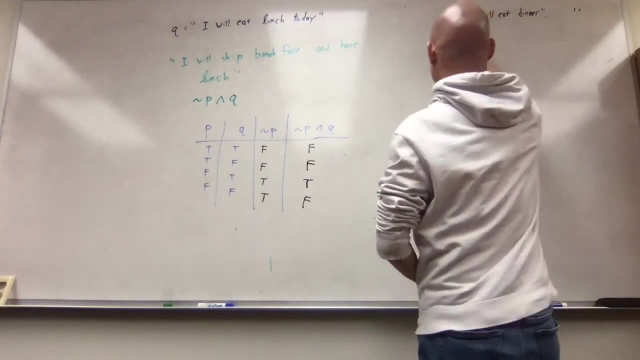 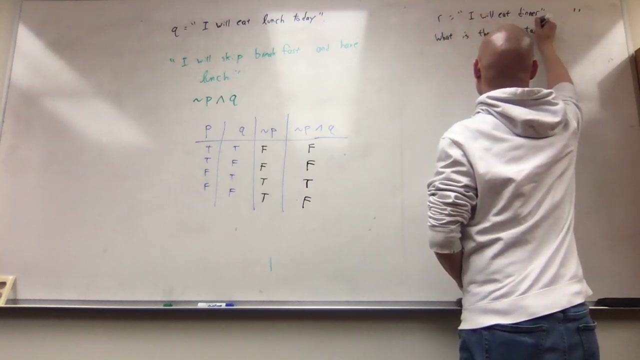 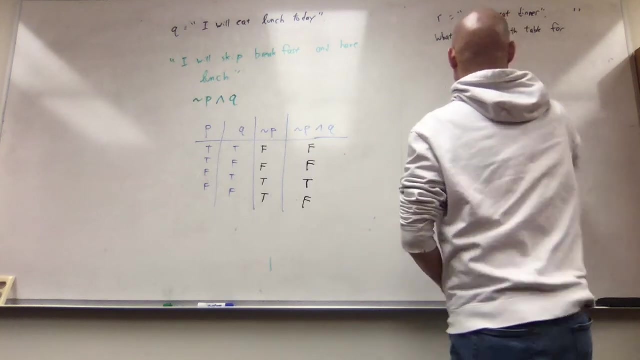 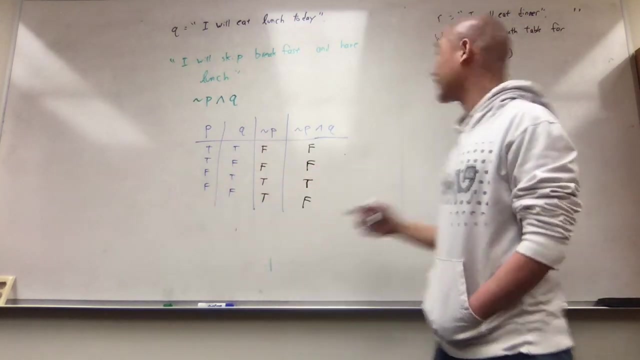 that. but again, at this point we should be moving past the need to attach a concrete value to our variables. so let's look at what is the truth. table for, for, for not p or q and r. so p could be two things, q could be two things. our new thing, r could be two things. so that's. 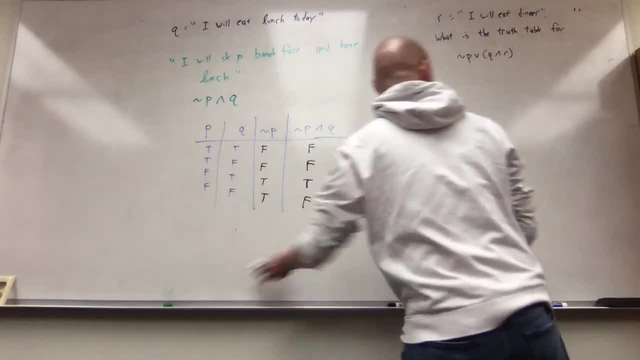 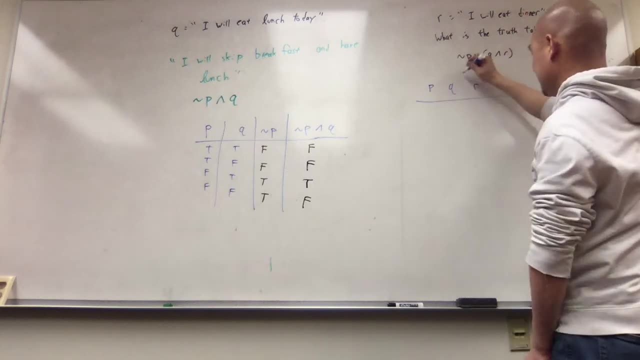 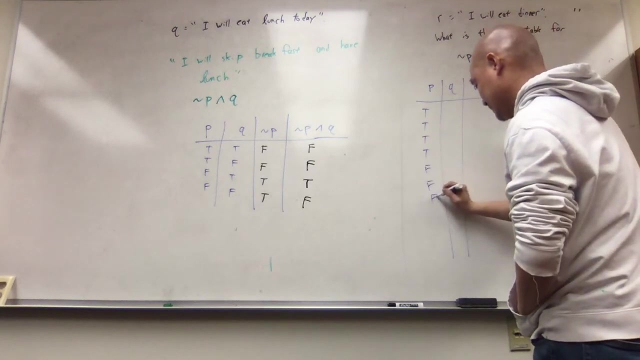 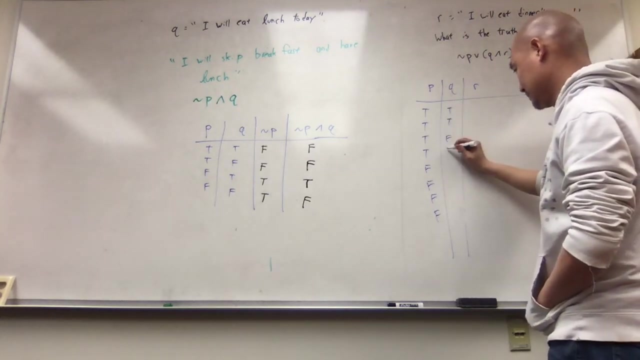 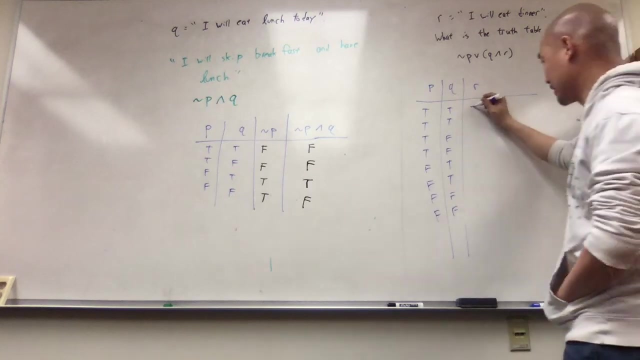 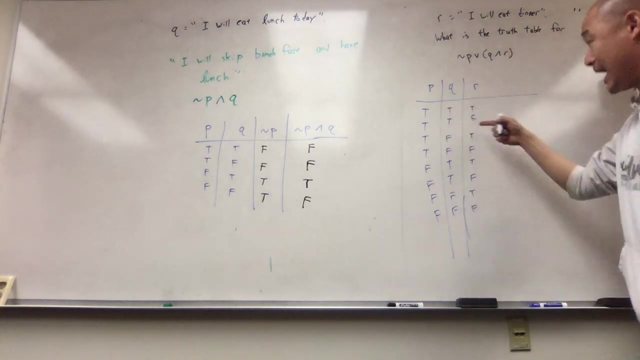 eight possible combinations: half the time p is true, half the time p is false, half the time q is true, half the time q is false, half the time r is true, half the time r is false. and you follow this pattern down, we see we have every possible combination of true and false. 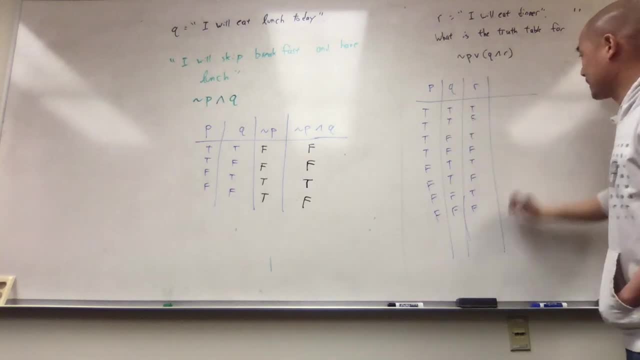 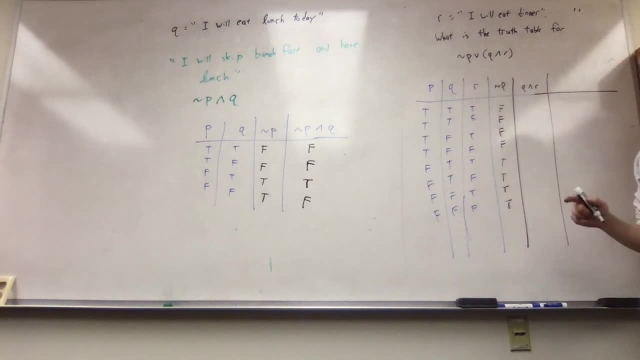 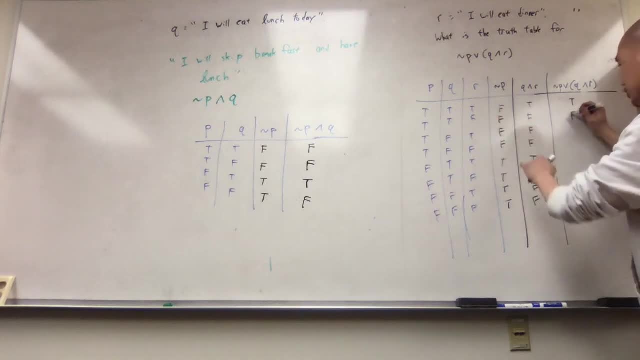 this one's true. true, they're both false, so false. they're both false, so false. they're both false, so false. they're both true, so true. this one's true, this one's true, this one's true. so this would be the truth table for not p or q and r. 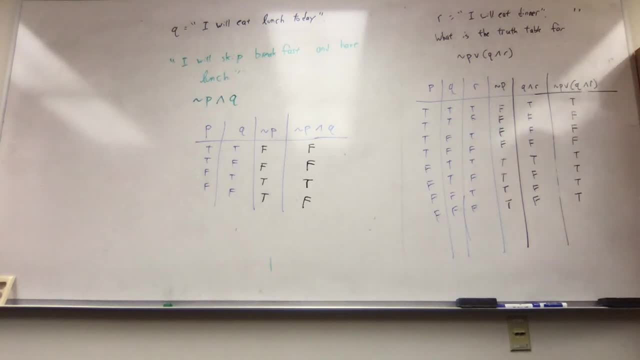 so, in the context of our meal examples, we could say that this is i'm going to. i better make sure i'm still in the range. okay, i think i'm still in there. i'm either going to skip breakfast or i'm gonna have lunch and dinner. right so if you have lunch and dinner, that's true, right so if you have? 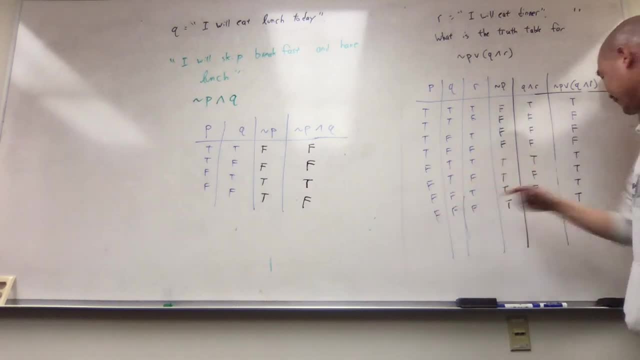 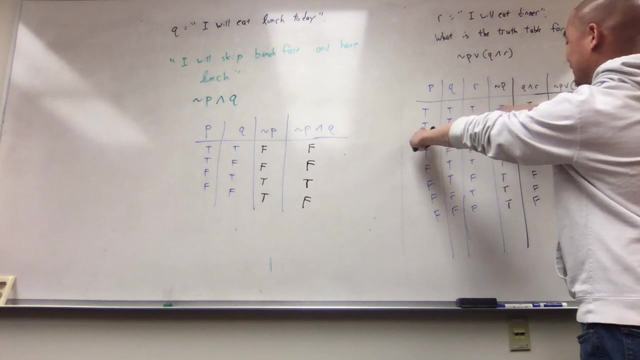 lunch and dinner, that's true. and if you skip breakfast, that's also true, right. but let's say you eat breakfast and you eat lunch, but you don't have dinner. well, you ate breakfast, so that's not true, right. you ate lunch, but you didn't have dinner, so that's not true either, right? these are. 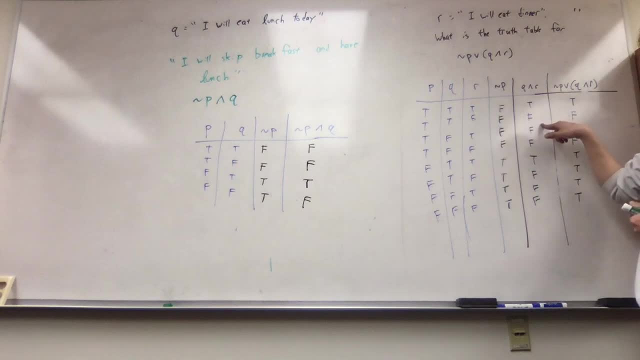 both false. you didn't skip breakfast, you didn't have both lunch and dinner, so your statement ultimately was false. all right, so i hope this was instructive and informative and that this will help you with your studies. again, if you have any questions, i'm happy to address them in. 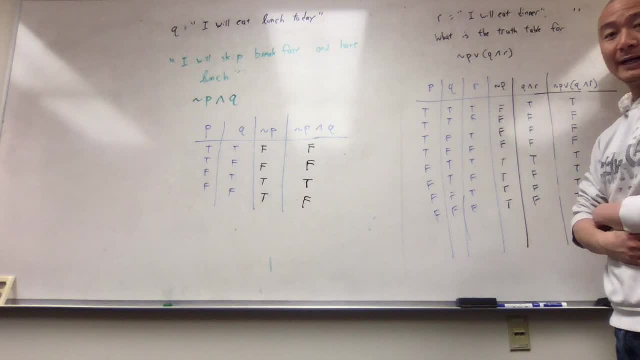 video form if you want, or you can always send me emails in the usual way and i'll send that back to you. um, byron, could you kill the recording? yep, thank you very much.